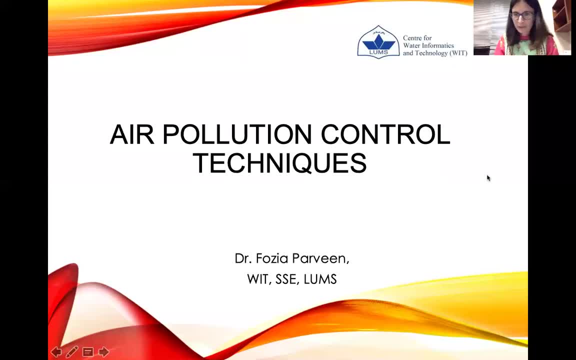 Great, So I hope that you are not too overwhelmed with all the experiences you know, not just for this course, but everything else. Like in last night, I realized that half of you have too many things on the table and you're really stressed with how things are going. 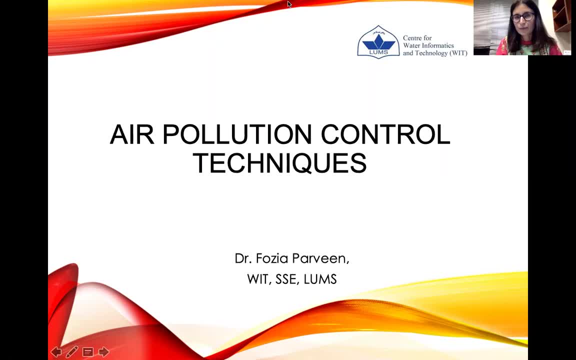 I would just recommend you to relax and do your best and then just wait for, I hope, a happy result. Today we're kind of discussing- I think these are the things that I kind of come back to, because I discussed them in chunks and I've kind of tried to give the solution right there. 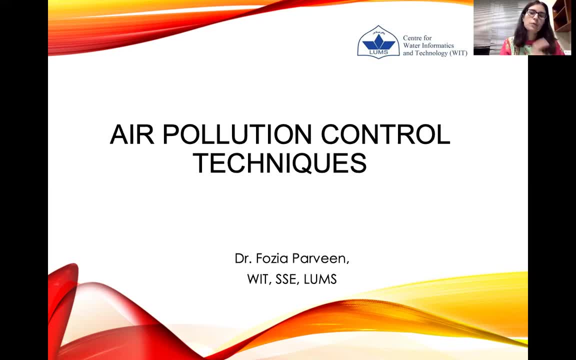 But when I speak with some of you, I realize that because I haven't put it under a certain title, you think that we haven't studied it, And I just wanted to bring all of this together to make sure that we now have a picture where we have overemphasized on the sources of pollution. 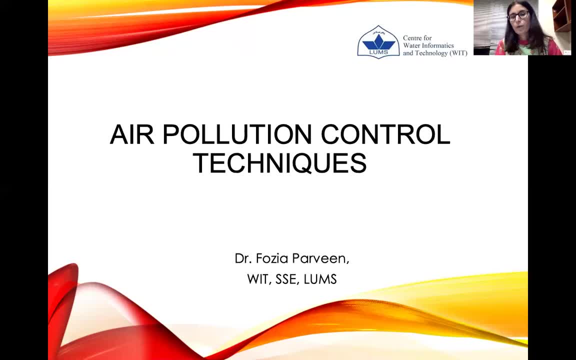 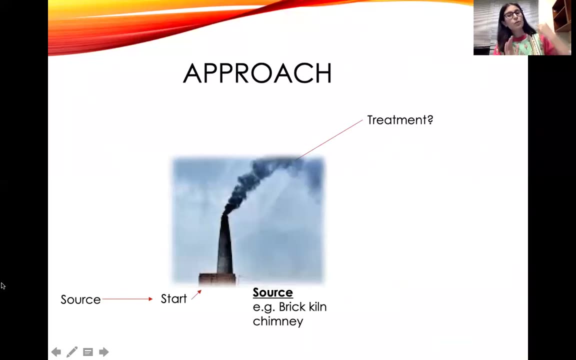 And now in this lecture we will kind of try and overemphasize on the sources to control or treat the pollutants that we've been talking about. And you know what would if you were somebody, and this question is for everyone. 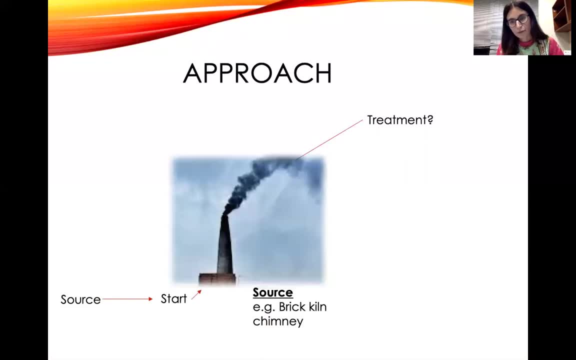 if you were somebody who had to take care of pollution, and this pollutant could not be air pollutant, only just think of any pollution form of pollution- How would you like? what would your approach to the treatment would be? So let's say there is a pollutant in the environment. 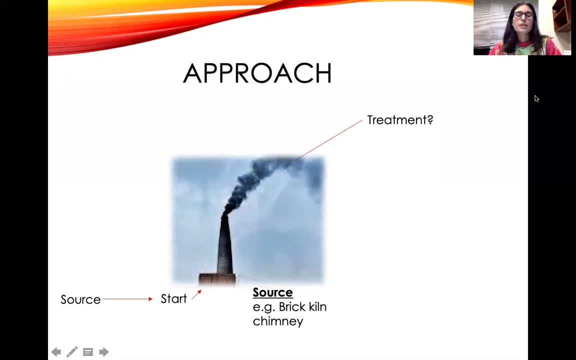 What will you do first if you want to get rid of that pollutant from the environment? Rafe, Yeah, I'll study its sources, where it comes from And how that can be prevented. Okay, Hasan, I think the first thing, after nailing down the source, would be to check whether, like let's say, we're making bricks, right? 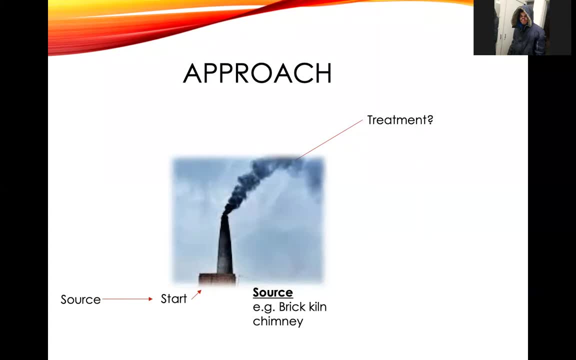 So I would check whether there are any alternatives available, whether we even have to produce that many bricks, Or is there some other way that we can also provide for, like construction material, Great And Manal Manal? I think assessing the damage is also very important. 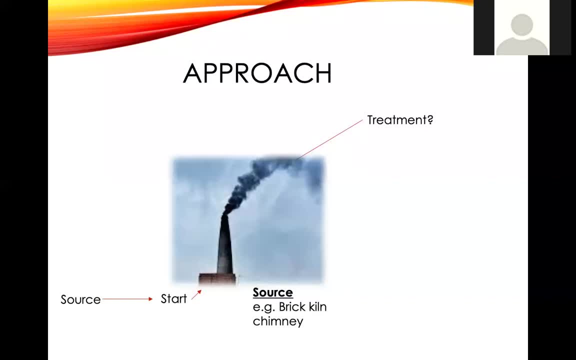 Like in the region, to see whether how much of it is reversible and how much of it is just completely hopeless. So I think assessing the extent of the damage is also very important. Yeah, That's correct. Somebody else has raised their hand. 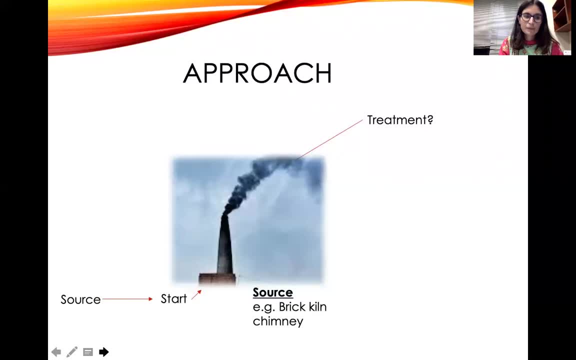 Ayman Rehman. Also like observing patterns, right, Because in certain areas there are certain kinds of pollution, right. So just like generally observing patterns really helps locating what the source is. Yeah, Taha. 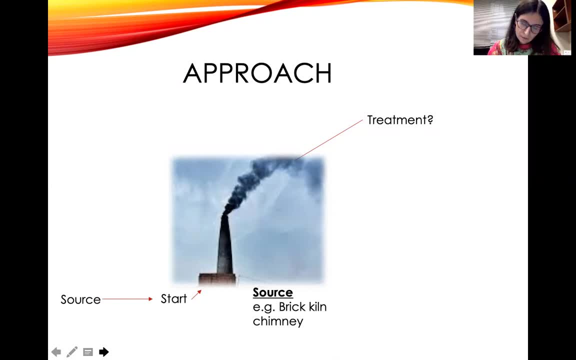 Another thing I think has some significance is that You also want to look at where exactly it is polluting at, Whether it's in the center of cities or whether it's in a far out area, How much of it affects people. regarding that: 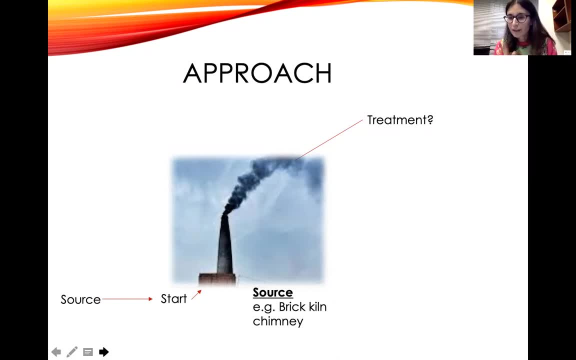 Great. So I think, sorry if I missed somebody and they had raised their hand early. Okay, Now you know you were all right And you know, of course, that would be a bigger exercise for us to think: what should we do first and how should we organize this? 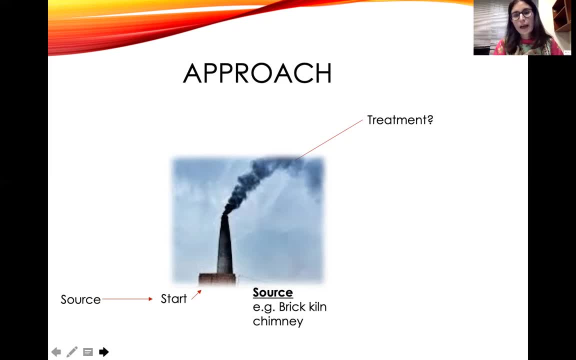 But let's say that I am a brick kiln owner And I am producing bricks at whatever numbers that are being expected of me. But there is a problem And that is that while I support some poor families in the process and produce bricks and, you know, make income for myself and others- the end of the pipe has pollutants. 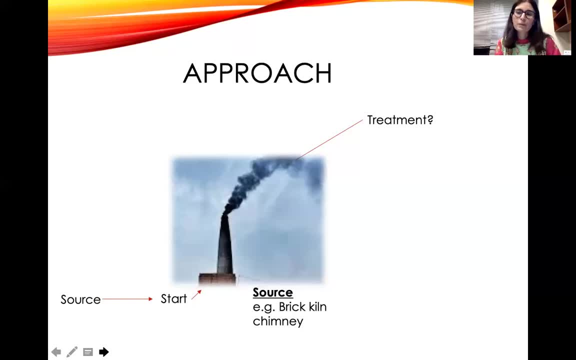 Now I want treatment for that pollutant. So let's say, in this case it's the smoke that is coming out of the stack, the chimney. So what should I do now? How should I treat it, Or what should I think? 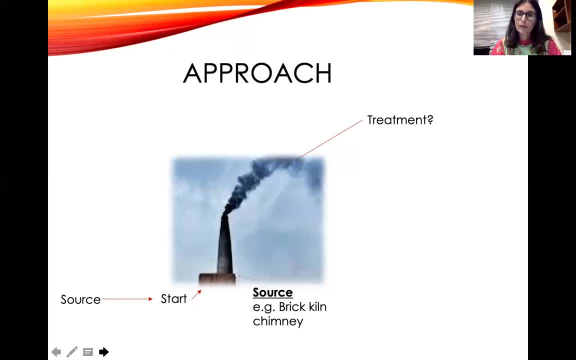 Like what should my thinking process be, Hamza? I mean like filter the air inside the chimney and then release it, Like that would be the best option. Yeah, So end of the pipe. This is called end of the pipe approach, right? 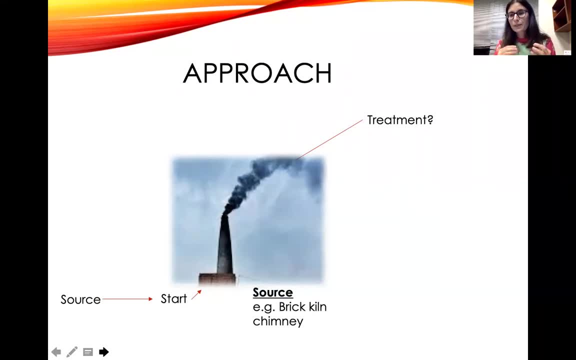 A lot of people say that when you are thinking to address pollution or solution for pollution, there are multiple ways to look at it. So if it is, let's say you know you have a pipe. So if it is a pollutant and source, for example, if we're talking about fossil fuels, you know here someone might have asked me: what is your source of fuel? 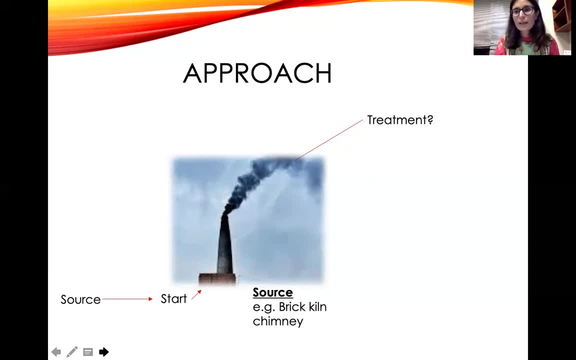 How do you fire the bricks, And maybe given me a proposed solution there, Someone else might have said OK, because you don't have an alternative to this. even if you're using clean fuel, you're still going to have some smoke in the air. 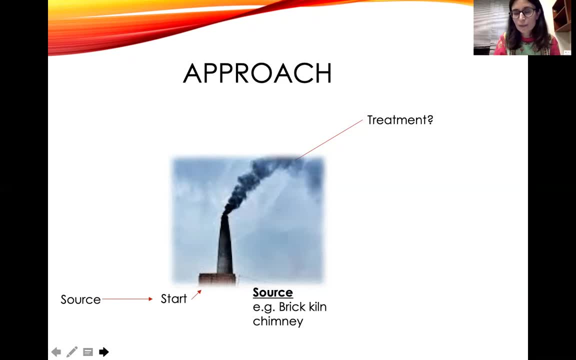 Or even if you don't have smoke, you're still going to release some, Some gases into the atmosphere. This is what you should do. But whatever we do, it has to be close to this source. You know it has to be close to whatever we are. 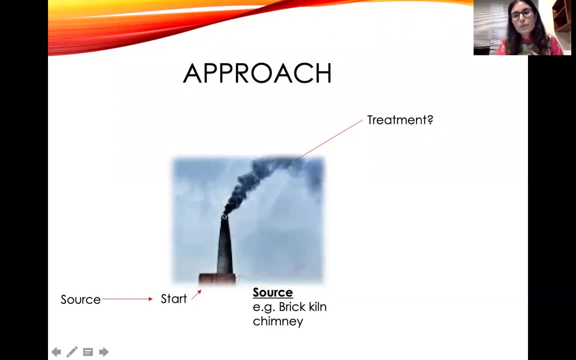 So if I am someone, if I'm in the government and I'm making decisions on how should we propose a solution to this, And I'm asking the funding body to, let's say, propose a treatment or cleaning of the air project miles away from these projects or miles away from this industry. 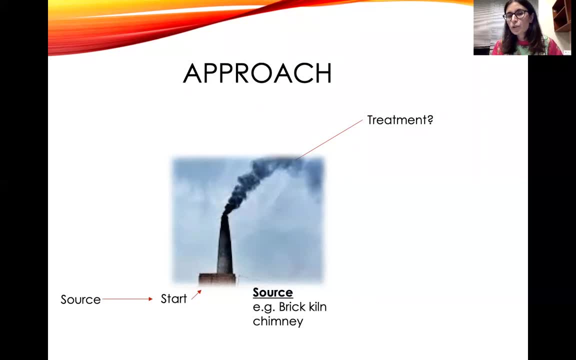 Then would that be wise. So I think there are a lot of those questions which you know. perhaps before science or with science, you need to ask yourself: is it the raw material, Is it the process, Is it the end of the pipe? 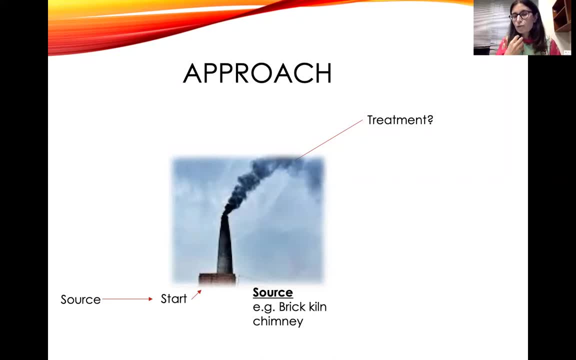 Is it the you know. you know how should you look at: getting rid of emissions and making source that you treat it, making sure that you treat it close to the source. So that's the approach you know. And in case of air pollutants, let's say if we are looking at. 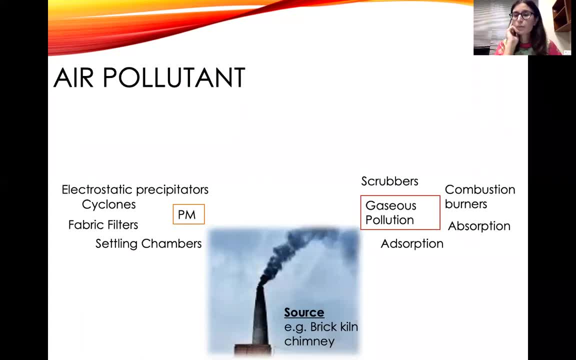 Looking at any Kind of pollutant, it's generally categorized into two and those two are either called gaseous pollutants or particulate matter that we've been studying a lot or at least mentioning a lot in a lot of our presentations. 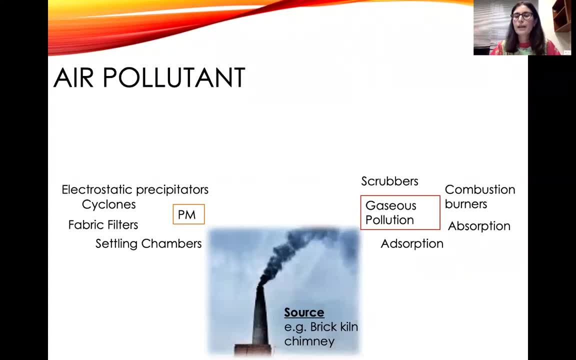 And there are various technology is already out there And I've mentioned some of these, but I'll still highlight some of these again today for you to kind of relook at what this is. So exactly what to place here. And maybe at some point, if we have time, we can do an activity where you propose a solution to one of these sources of smoke. 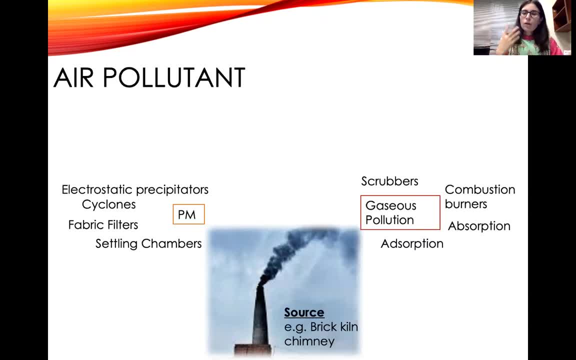 So what I've basically done is I've picked up all the sources of smoke that we discussed in one of our presentations, And I'm only thinking about those. These are perhaps more suitable for industrial setups or power plants or places that use excessive fossil fuels and have those infrastructure. 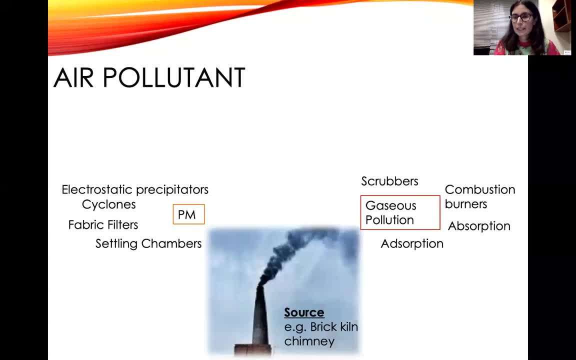 And that kind of technology that can facilitate this, But that doesn't stop us from from using these and others. Anyways, we categorizing air pollutants into particulate matter and gaseous pollution is a gaseous pollution, And we've already read them in our previous presentation. 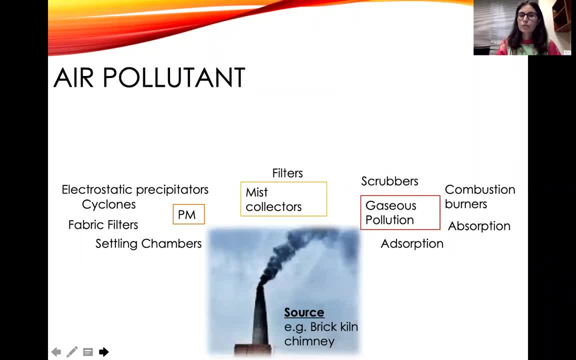 But there are now other categories that are emerging in. So, despite the scrubbers, absorbents- absorbents which we'll discuss in a while- you know, mist collectors generally come with the scrubbers or the filters, But they're also coming in separately as well. 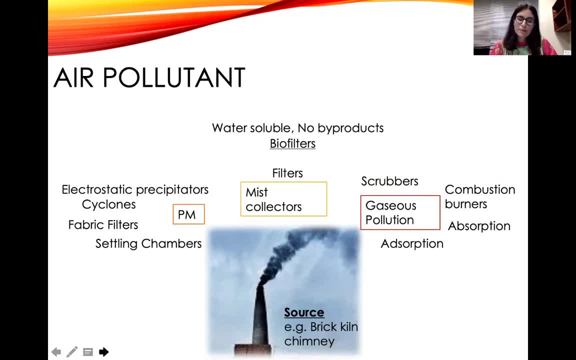 And something which is kind of more related to environment and environmental sciences is the bio based solution or nature based solution, And that's called bio filters, where you have a filtration process where microorganisms are also adding in into the process of degradation of the pollutant. 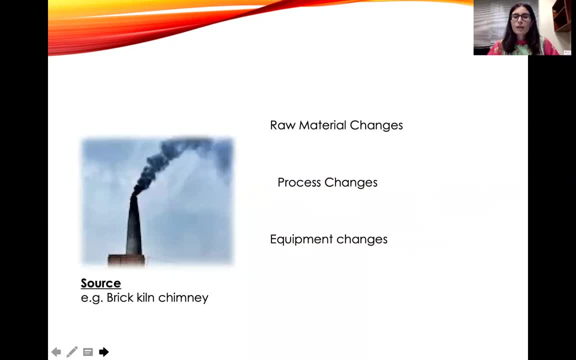 By the way, just to ask you guys, can you think of a pollutant And then think of how that would become, how it's harmful and how it would become less harmful? So let's say Yes, Iman. An example of a pollutant could be sulfur dioxide. 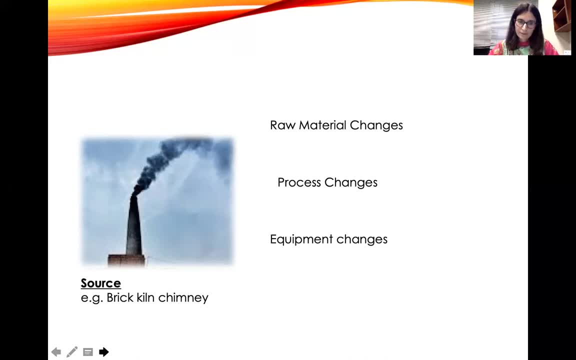 It's harmful because it can cause acid rain, and the way it could be reduced is through flue gas desulphurization, which is like you can in the chimneys you can put like a filter which scrubs the sulfur dioxide, making it less harmful. 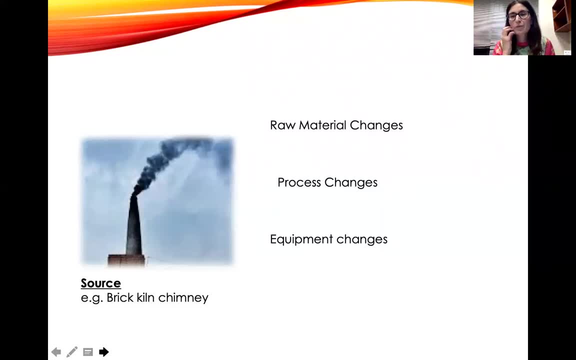 Great Yeah, Amazing Yeah, But that's what we'll. these are the things that we look at, Right? So what are we using? Are we using any chemical form? What is the chemical doing to the sulfur? How is it reacting with it? 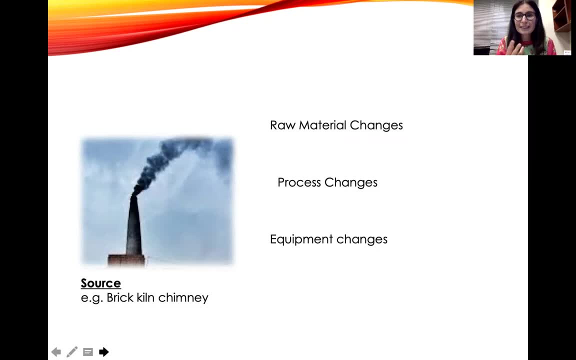 What is it turning it into? You know those, those, those questions, But this time we'll give it a name. Is sulfur dioxide reacting with lime? What is lime? And then, what will be the final product, and how, how that is less harmful than the original product. 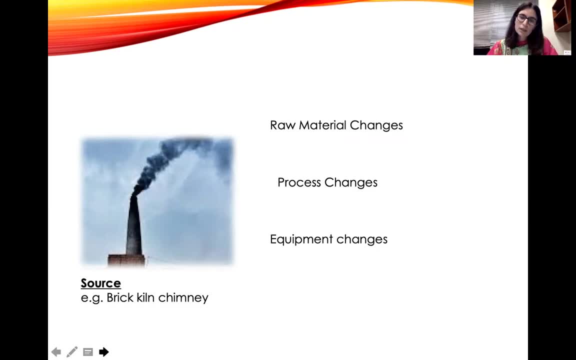 Aman, you have a point I am. in this kind of smog There is a large concentration of carbon And recently I visited the factory side of Lahore And I saw there that a man was smoking in the back of his factory. 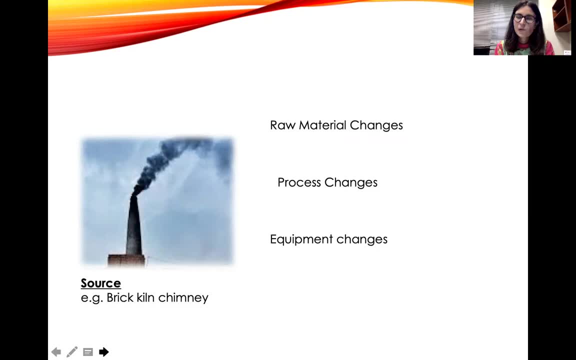 He had covered this chimney with a wall. So I asked him the reason. He said that the carbon waste is going into the air, So it will be stored in the room And then it will be reused And the remaining gas will be removed from the site. 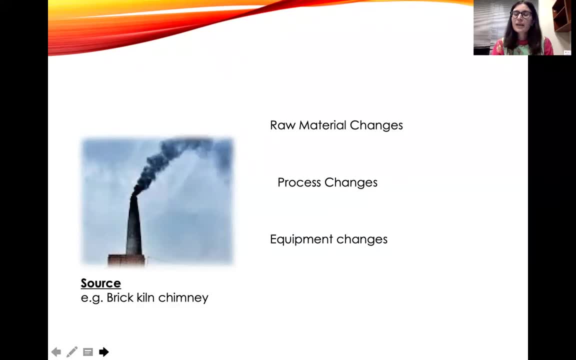 So we can reuse the carbon in this smog. How many of you had the time to look at the video that I sent you? Did anyone manage to? I want to ask somebody new Iqra. Okay, so that video. I don't know who was the guy. 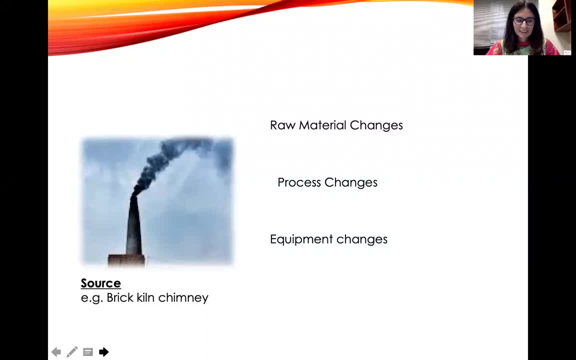 He told that he was trying to solve the problem of smog. He said: there is so much smog and we are industrializing. We are increasing our industries and oil in China. There is so much manufacturing But our air is not clean. 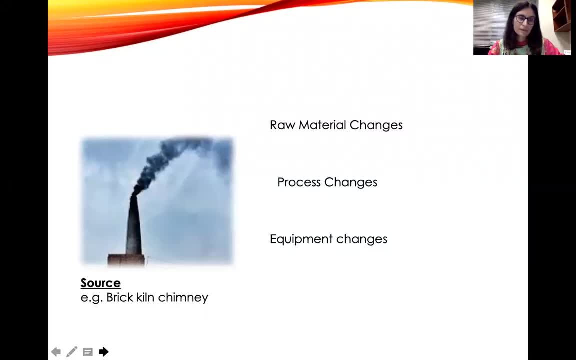 So how we can clean the air and what initiatives we can do. So he thought an initiative that a filter which can take the air, suck the air And absorb all the carbon and release the clean air to the environment. And after two years, 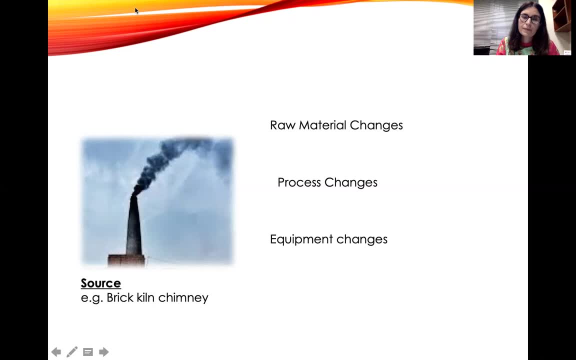 He developed the large filter And placed it at the part where he Where the air goes in a filter In an yellow scale And by using the electricity which is around water boiler And with the positive ions, And release all the clean air to the environment. 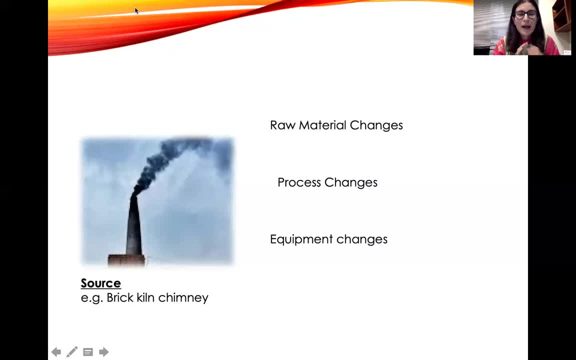 So, yeah, Okay, I was in the audience when he gave that talk And I think in that one hour lecture that he gave, He probably taught me more than most of the teachers who have taught me in my courses- And this is with all due respect to the teachers. 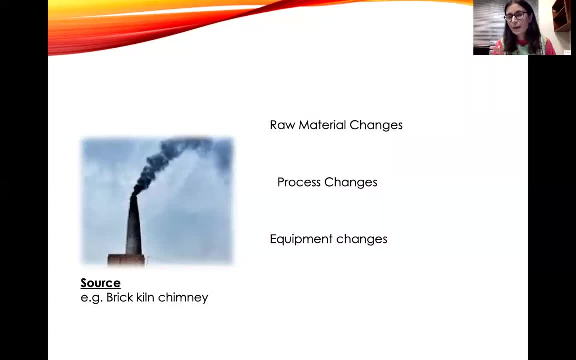 But I think the way he said it And the way he thought, And again, I think this is why I keep encouraging all of you to think about the environment, Because he's an artist, So he just thought about the possibilities, Thought about design. 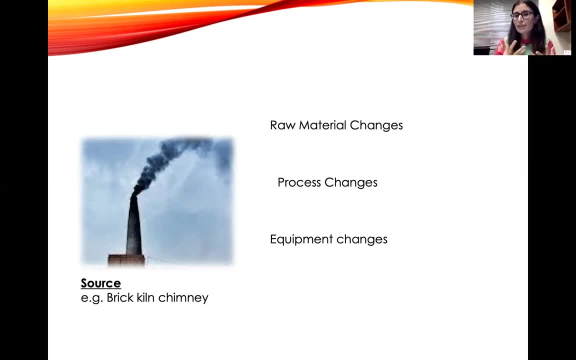 And then, you know, talked to people, Talked to scientists, Just gave a wild idea And threw it to many scientists and engineers And some of them said this is possible And he eventually was able to do it, Which was basically just hoovering the air. 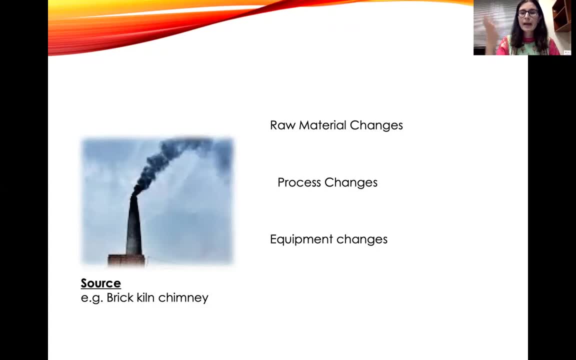 So just how you hoover the carpet, He was basically hoovering the air And kind of getting the smog And at that point I think instantly it was a great solution And also thinking that he was creating those. You know how people say that when the air is not clean. 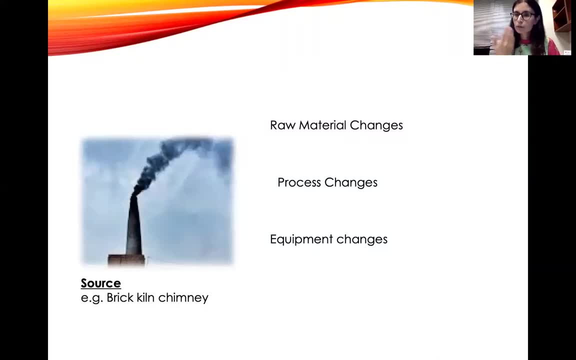 Even if you're going to the park, It's not really good for your health Because you're still taking in all of that smog. But he was, by putting these filters, Creating those spaces which were more clean than the rest of the city. 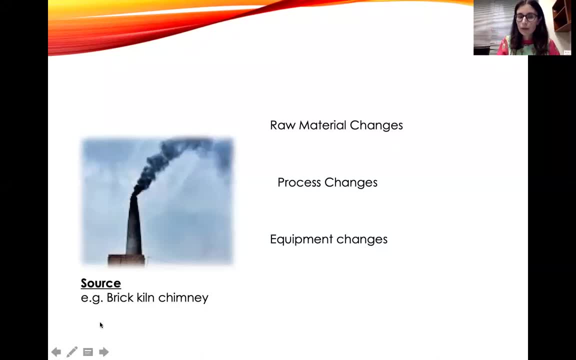 So automatically it became that public space for everyone To come and enjoy, With 100% guarantee That they will have better air than the rest of the city, And then also contributing to the city After the project had finished or evolved, To buy all of those products that were made from that compressed carbon. 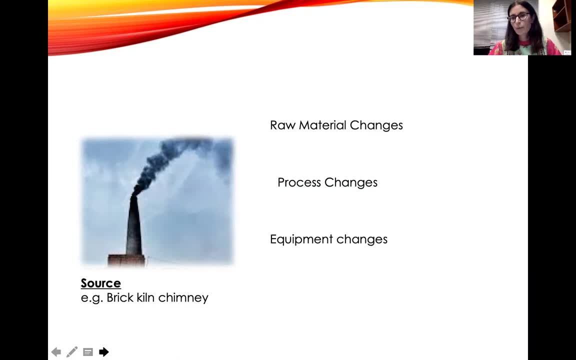 So I think it was really interesting. It really inspired me. I hope you took out something from it as well, But I would really encourage you to watch the entire video, Because there are a lot of other things that he's doing That might interest you as well. 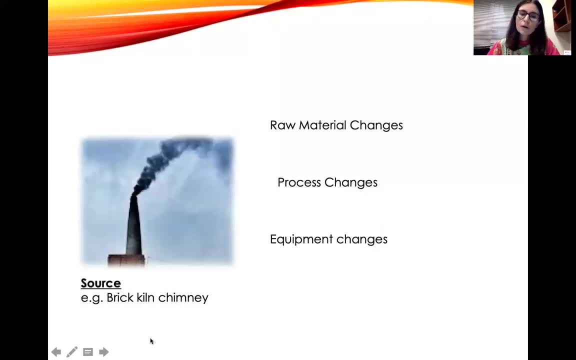 Because the discussion is going to be majorly smog and smog oriented. I thought you should watch minute 10 to 20.. All right, So we just had this discussion To reduce pollution. We will think about either changing the raw material. 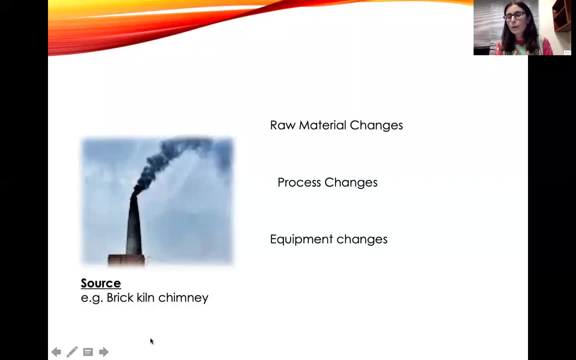 We will think about changing the process. Is there anything that's wrong with the way we're doing things? And there is something that you know: the process has changed For brick and industry recently in Pakistan and India, And I'll give you the task to look up what that is. 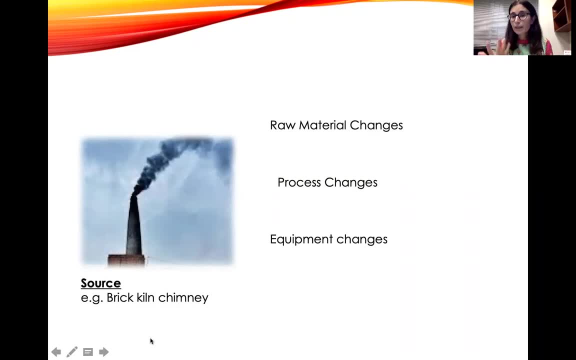 And then, past that, of course, as Hamza said, We can think about changing the equipment, Bringing in more efficient equipment, Bringing in pollution control equipment That are already designed, That are already present in the market. So it's not like you have to design and innovate something yourself. 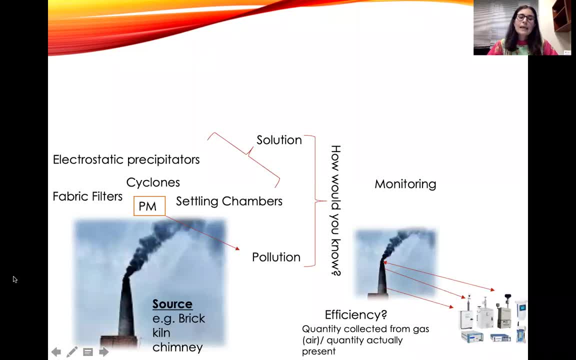 All right, And so let's say that we have all of these particulate matter in the air And that's the pollution. And there are various gadgets available in the environment, Such as electrostatic presses Or the air purifier Or the air purifier. 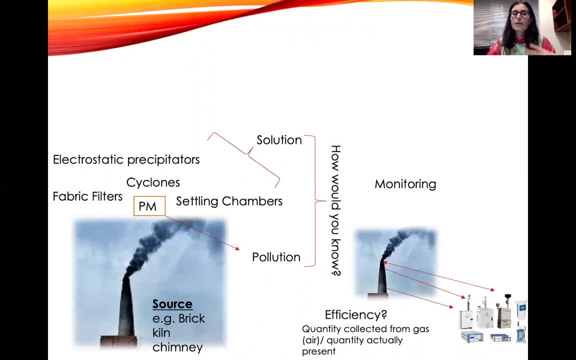 And the other thing is, you know You can have a lot of other things Like precipitators, cyclones, filter bags, settling chambers Which can get rid of that particular matter In your indoor environment or in the air Then, but how do you know? 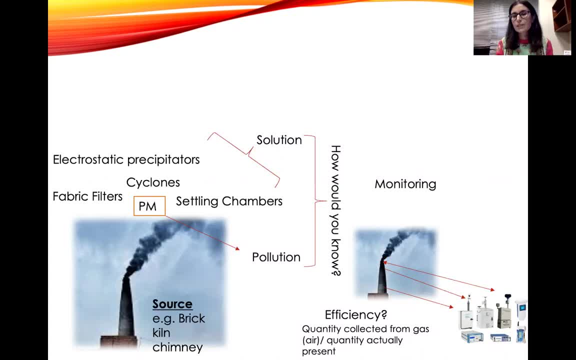 That This is the technology that's doing it for you. So I think something that I haven't really talked in detail to you but I would still like to mention Is the fact that you know you, you would still check the efficiency. 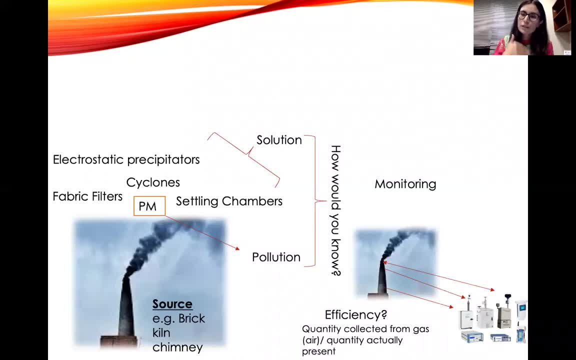 It's not like you put a gadget on and you say: this is it. You have to do. You have to continuously monitor it to see that it's actually reducing What it says it's. it's reducing whether that's a. 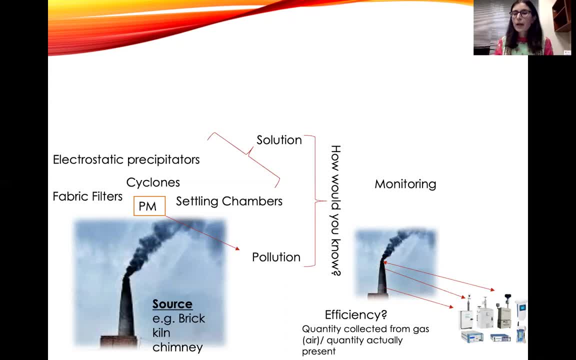 Particulate matter, 2.5 or even below, And to do that you would Put certain gadgets on, get the quantity From you, know what actually was in the air And then what you have after you put that gadget. 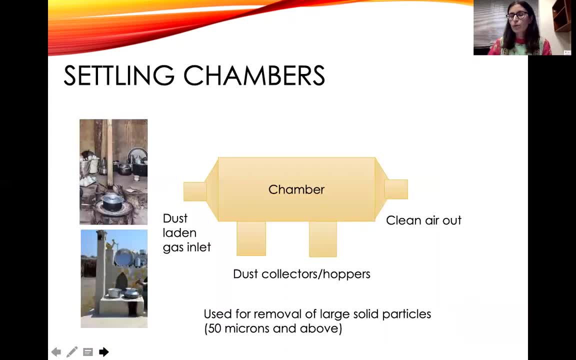 So it's, it's just for you to To know that you can go beyond this as well, And This You can see, And then you can just, You can just You can just come back In and And that's it. 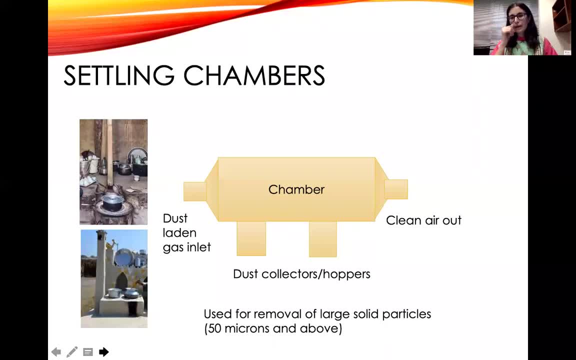 Cool. So we're going to start with setting. Does anyone, does anyone want to guess what it is? because it's very straight away: Treatment technology for air. So let's say that there's an air Which is Smock Or particulate matter. 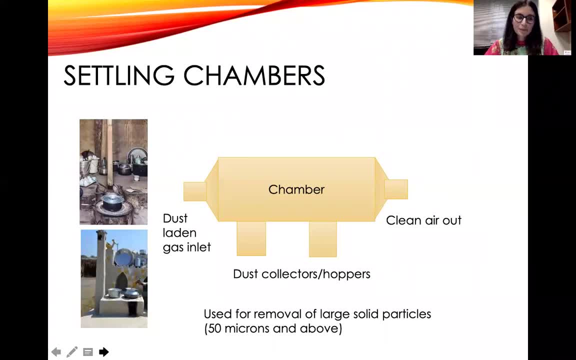 And And you put a setting chamber. Not Yeah, I See In the picture, I can, I can get. So It's, It's, It's gas. so basically, when we burn things out, okay, so they do our smoke, so they create these long. 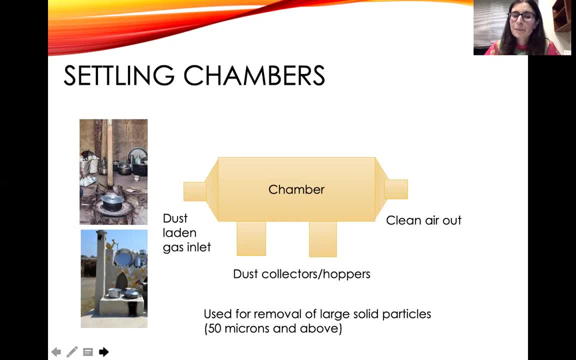 chambers where the particulate matter just set and settles down or it sticks to the linings of the chamber so they create a particular, we can reduce the amount of particulate matter that we can send out to the mix with the smoke. yeah, so if you're basically using the concept of gravity? 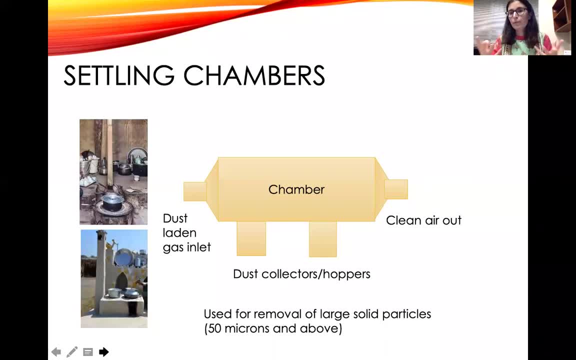 because the if it's, if it weighs, if it's weighs enough, and you are not allowing it to interact with the air, so that the air just takes it away at the source. you have provided this chamber. of course, this can be a simple pipe that you put at the end of your store in the north or in the south. 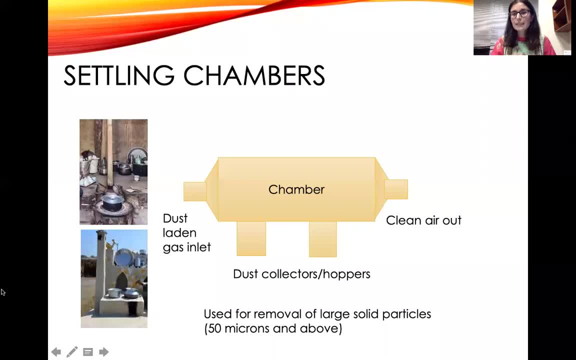 or it could be a proper chamber that's put in the industry. so let's say the particulate matter is really high. i once went to a miller mine factory, so you know miller mines used to make these um crockery close to plastic. i went there and i want to look at their health and safety condition. 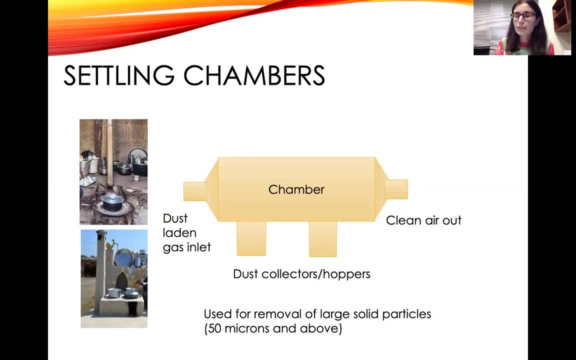 and i went there and the air was just filled with particles because they're using all of those gadgets in a small factory in pindi. it was just filled with dust, you know, and it was definitely above uh 50 micron, because it was absolutely visible to the eye, was big enough, it was settling. 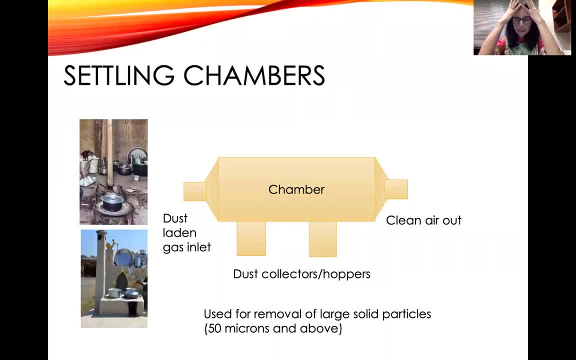 but for that short period of time it was staying in the air and all they were all covered from head to toe in in that uh, middle section of the chamber. that's where the air was coming from. so that's why it's called the miller mine dust or the miller mine raw product, uh, powder and um, and. 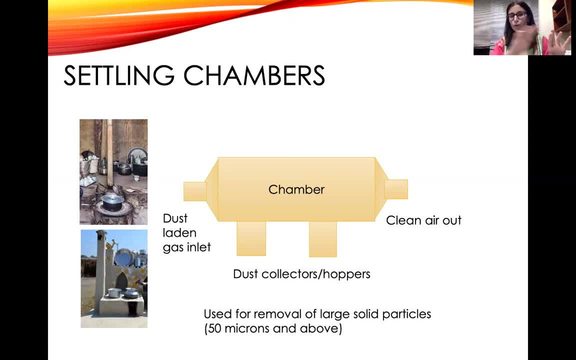 you know, those kind of things can easily be directed to a pipe or or then to a gravitational settler or a settling chamber where you allow the gravity to, to kind of collect it or give it the time to settle through gravity, and then at the end you have these dust collectors or um hoopers as 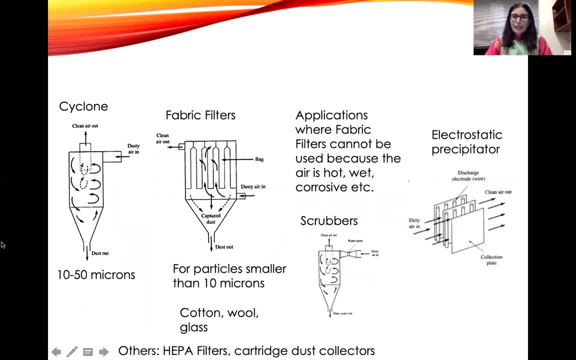 you call them in the industrial terms. quickly again, if anyone of you knows anything about any of these and would like to talk um, you're more than welcome. before i talk about cyclones, maybe i can talk about electrostatic precipitators. so do two things. can i talk about it? 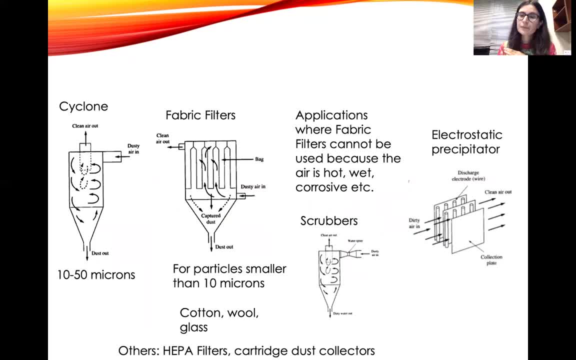 go ahead. yeah, so uh i in the previous side i was all, i had my hand raised and i was going to talk about the same thing. i came across a similar technology in which, like uh in in the breakers, in the chimneys of the breaking uh kings, they had like uh, they had. 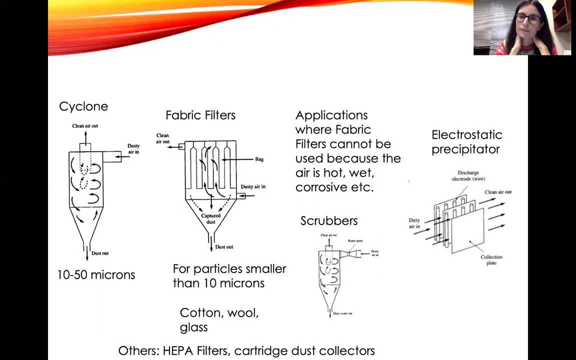 some technology through which they like gave a negative charge to the, to the uh sulfate oxides and and, and nitrate oxide and nitrates. and while they were like leaving the chimneys, there were these cathode trays which uh, which were positively charged, and these attracted these negatively. 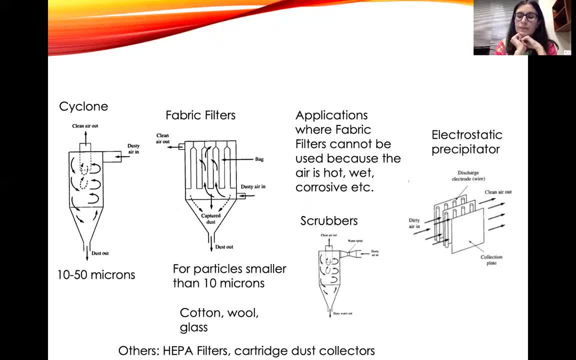 charged particles. so this reduced the amount of like of these oxides in the air by 90 percent and they they would, and this used to stick with these plates and later they could like easily wash them off from those. absolutely so who is basically? this is the simple. remember when you. 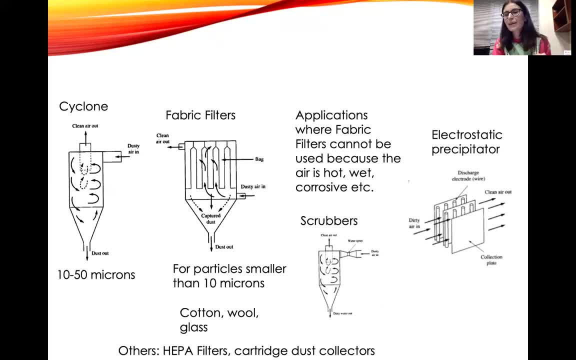 were all kids and we just used to take a balloon and then rub it against our clothes and then put it and it would stick to the wall. does anybody remember it? raise your hands if you know, if you've done it. just raise your hand so that I know that you're. you had a proper childhood. well, you a lot. 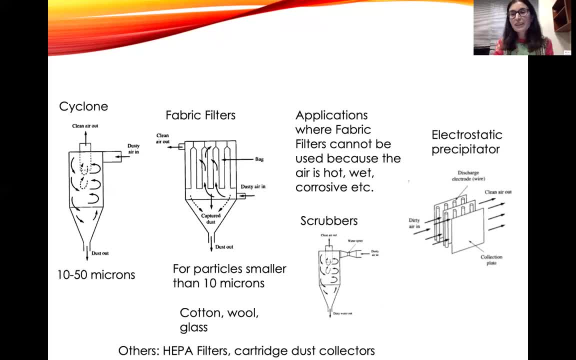 of you had a proper childhood. that's great. what were you doing there? that was absolute science, right? you were creating static charge, and that's why that balloon was able to stick to the wall. all right, and that's what you do at the electricity for the electrostatic precipitators as well, or in 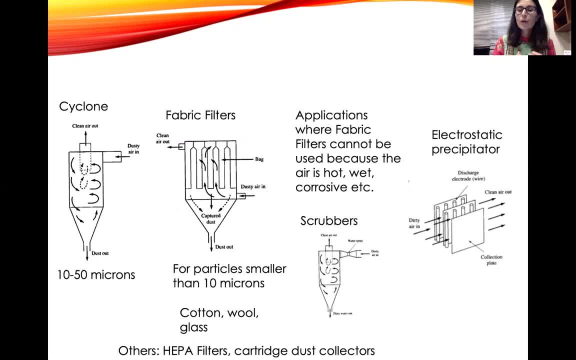 the electrostatic pressure precipitators. that same principle is used where you have the negatively charged rods that create that static charge, which so give a negative charge to the particulate matter, and then ahead of it you have cathode, which then allows the the particulate matter because it's 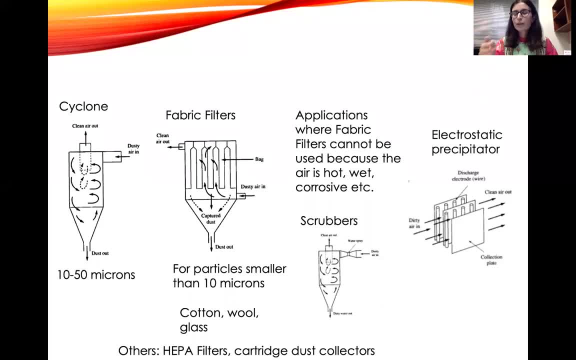 charged to go and stick to it and then clean air would filter out. so of course, someone who had developed it might have developed it with that same simple concept as well. you know how you can solve it with that same simple concept from the childhood to then bring it to solving worlds. air. 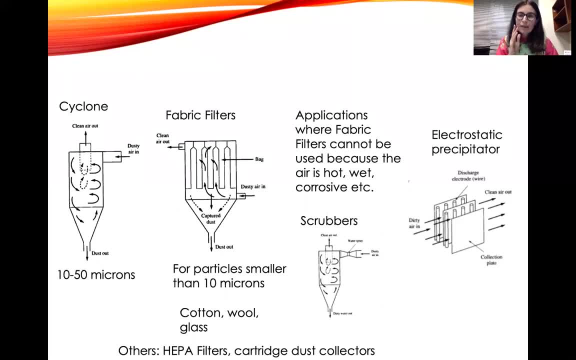 problem and then so. so that's that if you have any questions, if you don't understand anything you want to discuss more, raise your hands and let me know. there's a lot. I'm not talking a lot about the design. I'm not talking a lot about the applications, because I think, and the advantages, 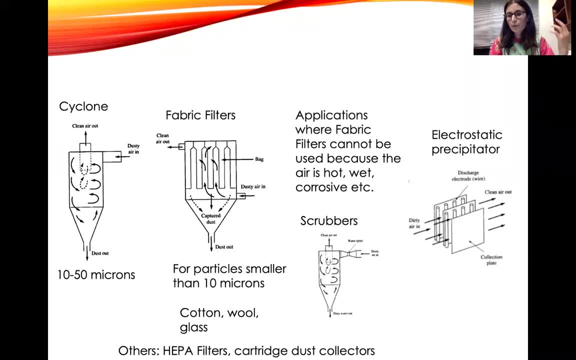 and disadvantages and the costs, because I think they'll waste a lot of time. so I'll just talk about the working principle and and then we'll see another slide in the next few minutes, but I hope the questions have been pineapple learning. the idea was awesome. it's been a lot of fun and amazing work. 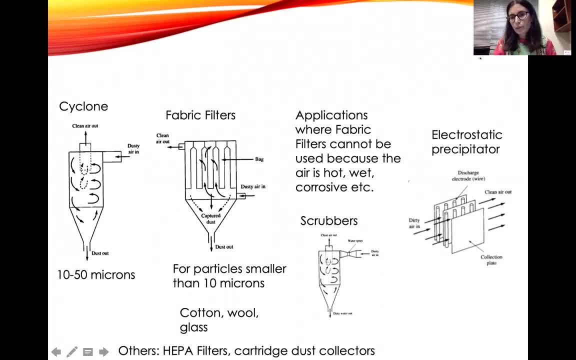 um, and then we we can go ahead. now do you have a question i just wanted to confirm, like: to what extent do we need to know these terms? i mean, i really don't, didn't understand this electrostatic precipitation process. so do we need to go over um ourselves, or you're going to expand on? 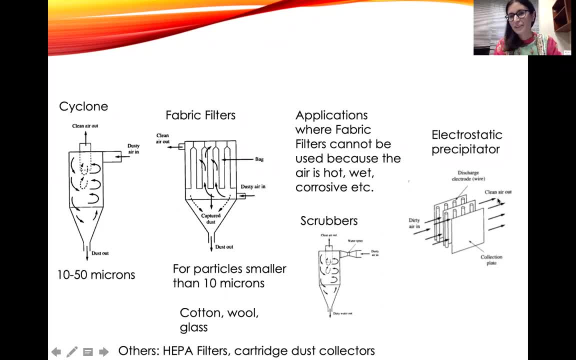 that i'll extend, i'll expand a little more on it, okay, okay, so what about fabric filters? there's a very there's a. there's a gadget in your house that i have also mentioned in the presentation that uses fabric filter and you use it kind of every day in your house or every other day. 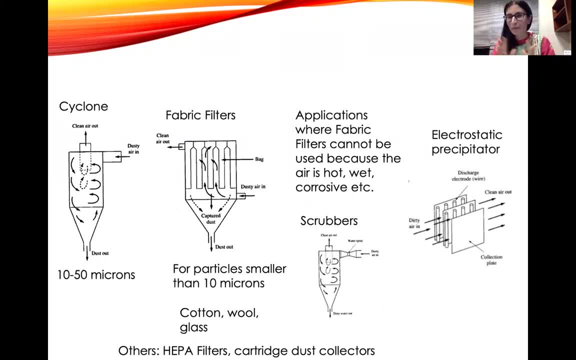 in the house. does anyone know where, in which particular home application, do you have a fabric filter for cleaning purposes? okay, how many of you say about ma'am? is it in, like the vacuum cleaners that we use? yes, it is the vacuum cleaner, so if you have never opened it and looked, 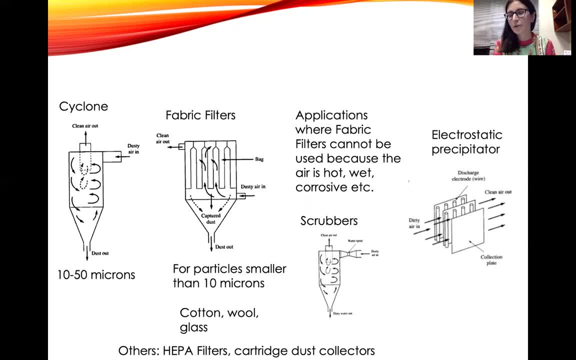 at what's inside and you know, if you've never wondered how, how it works, if you've never really looked at it, today is the day, or maybe tomorrow morning you can just help your mothers or your maids help the house clean the house. just take the. 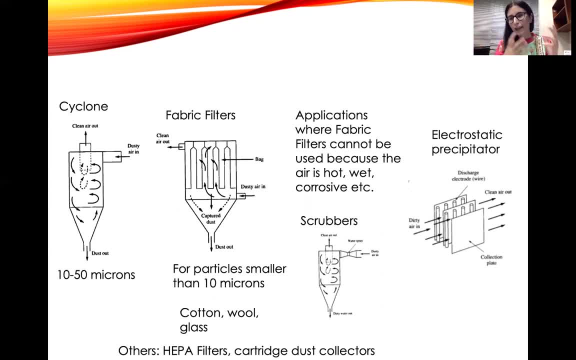 hoover open it, see all the components, clean it, look at how the filter bag is, and basically that's the principle which is also applied in the industrial application, where you're allowing the air that contains dust to go in and then kind of filtering the the air out and then 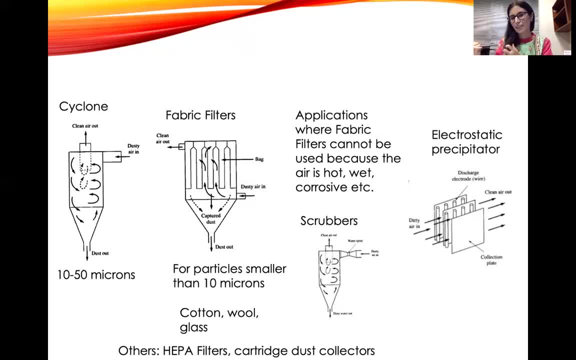 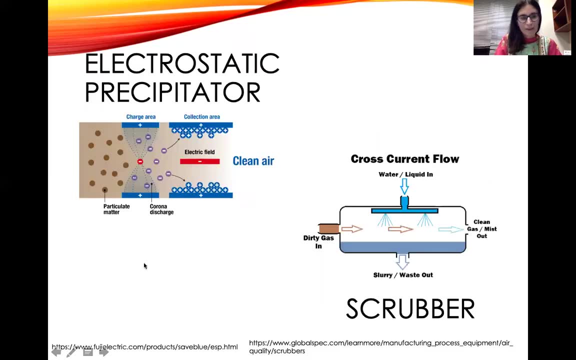 capture the dust and that dust is contained in that filter bag and you just take it. take it home. um, vacuum cleaners, okay, um, all right, uh, and then also there's the cyclone, so all of these are going to be cleaning containers that we use to have the air out. There we go, and then we also have the cyclone. so all of these are going to be cleaning and anything else that you use is going to be needed. And now i need to filter the filter bag and then, when you're returning the dust onto your pack and when you're coming out and say, hey, are you going to get it out and do things? how about this? 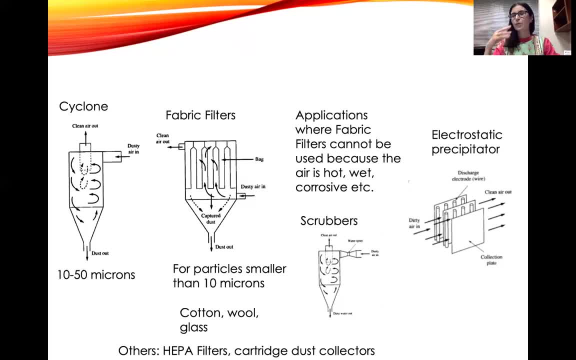 just you know, you would always look at them as machines. um, you wouldn't really know what's inside, but the working principle, i think, is important. if you don't know that then there's no point in knowing the names. um, cyclones again is where you, with the dirty air is going in with a particulate 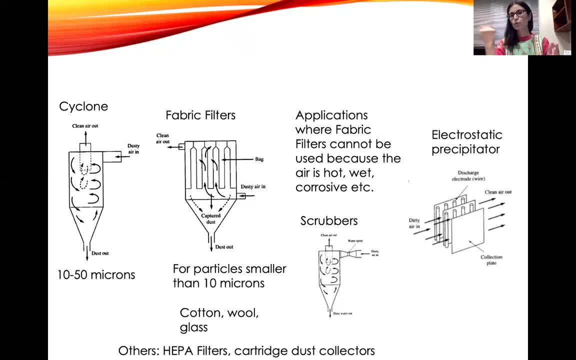 matter. you're allowing the centrifugal force, so you're like allowing it to travel whirlwind, and then when the particles hit the wall, um, they, they slow down and then they go and settle, um, so. so that's what's happening here, and- and i think the the arrows kind of help you through that as well- 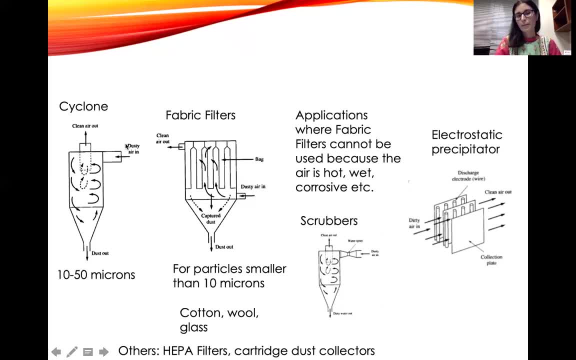 that the dust is settling down, the cleaner is going in, uh, going up, um, and everything else. i think is pretty, pretty clear, uh, but as you saw this, the settling chambers had higher micron sizes and then, as you go further up, the micron size will go down, um, so, um, there's another graph that we'll. 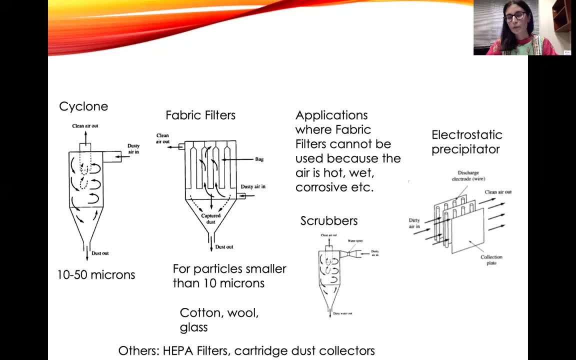 see, but um, before that i would like to discuss scrubbers as well. so up until now, other than the um, bioremediation or something like that, so do you think there are any? you know certain types of plants or organisms that can be planted near, like the soil or the soil surface, so i think that's. 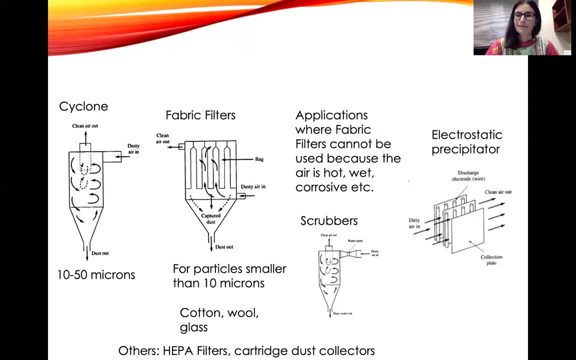 something that we're going to be talking about. but i think that's something that we're going to be talking about, but i think that's something that we're going to talk about- the site um, from where the um, you know, pollution is being excreted to like sort of you know. 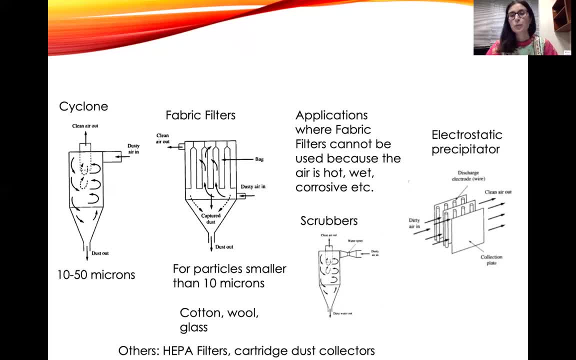 mitigate the effect. yes, yes, absolutely so, both for indoor and outdoor environments. the first thing that you ever ask any urbanization planner would be: please put trees on the roadside, and that's exactly the principle. so the principle would be for them to kind of absorb as many pollutants as 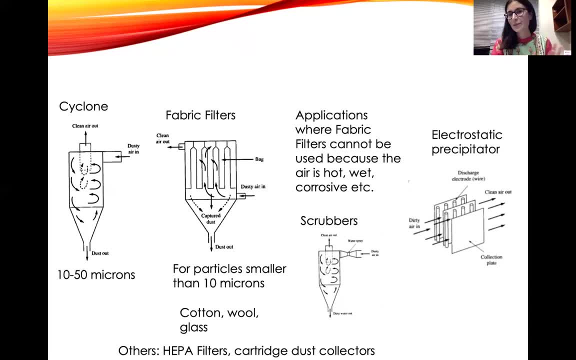 they as they can, but there's a downside to that. so we'll be discussing the bio filtration part of the air as well in some of the later slides. uh, but yeah and and they're quite clear. so if you just google, like, what kind of plants should i keep in the home, if for cleaning the air and similarly- 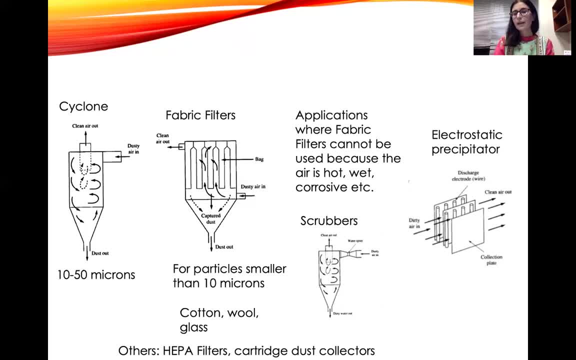 what kind of plants should be putting the in the environment. yeah, i mean, i have mixed feelings about it, but but i'll leave that for that, um, but then, after all of these, so it's, it's very simple. i think you need to summarize it because i i feel like i've made it slightly difficult for you to. 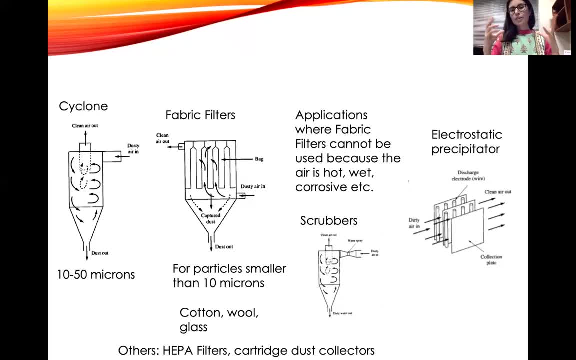 to understand it. so the particles are large in size or they can be very small in size. in the industry, the particles can be a nuisance. so it depends on what they are and it depends on what they contain and we want to contain it as a, as a man said, it can be something valuable. it can be a carbon particle, it can be a. 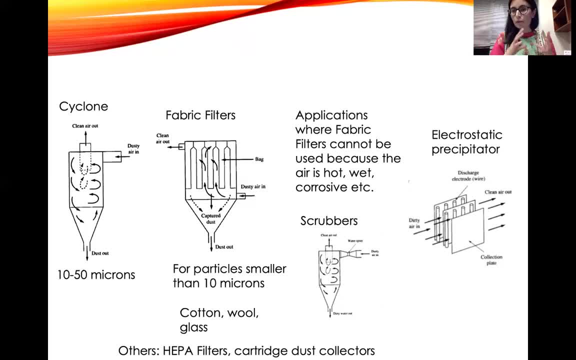 suit, it can be something else that perhaps is a resource for that particular industry. so a lot of industries actually captured it because that waste particle or suit is a resource for them. some capture it because it's a nuisance and they do not want to create harmful impacts on the environment. so if the particle is bigger they could just go. 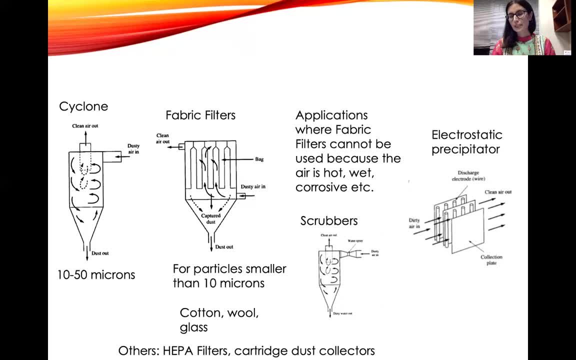 with giving them that chamber, which would allow them to settle um over the settling chamber using gravity. or they could just give that air current um, use the centrifugal force so allow the particles to hit the wall of a cyclone and then slow down and then eventually settle. or they could just use 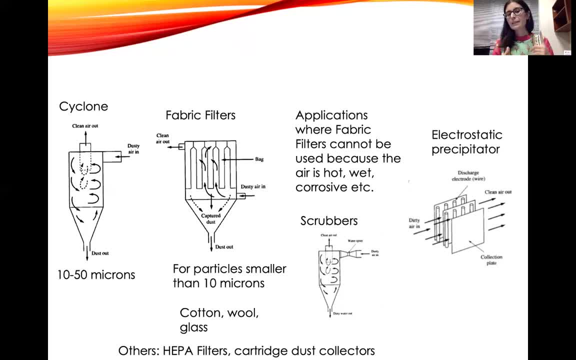 a filter. mostly fabric filters are used. there can be glass and wool and cotton and all kinds of fabrics as well. depends on what kind of strength do you want and what kind of characteristics do you want, because some chemicals can can damage the fabric. so let's say you're just simply filtering out exactly how you filter your clean water. 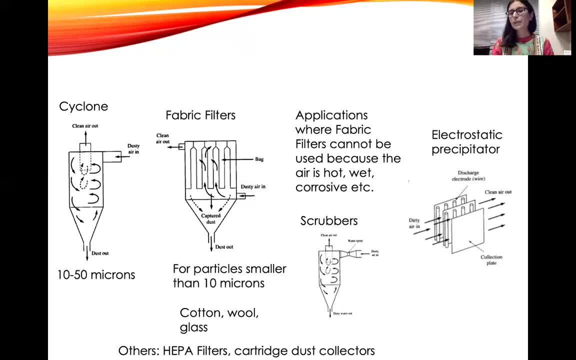 your, your boiled water out, but this is a different kind of fabric. it's it's smaller, uh, pole size, um. so that's that, and then um, electrostatic precipitators. as we said, it's basically charging the particulate matter. so the particulate matter is inert, it doesn't have a charge, it's not just. 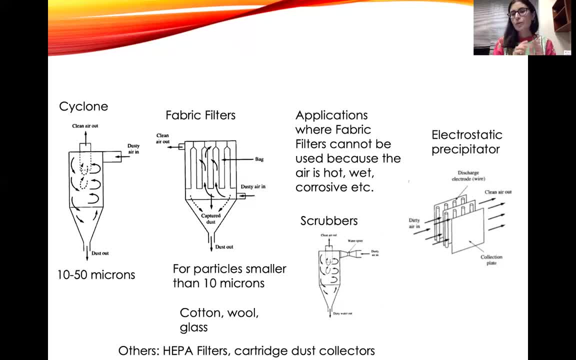 there you are, optim, you're giving it a static charge, um, and the static charge meaning you are, you know, waking it up, um and and telling it to, to to have the charges towards outside. basically, i think the balloon is a better example. so, just like the, you're asking a balloon to charge, develop the. 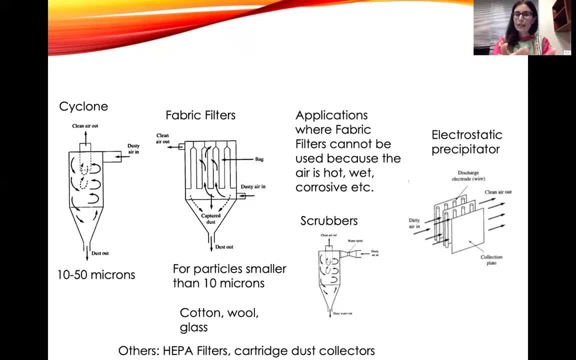 charge statistic, statically, so that you can then create a little bit of energy for the particulate matter and then you can, um, you can, then you can take care of that particular uh plate that could take care of that particular uh particulate matter, and then the clean air goes out. but all um particulate matters are not that easy, it's not. 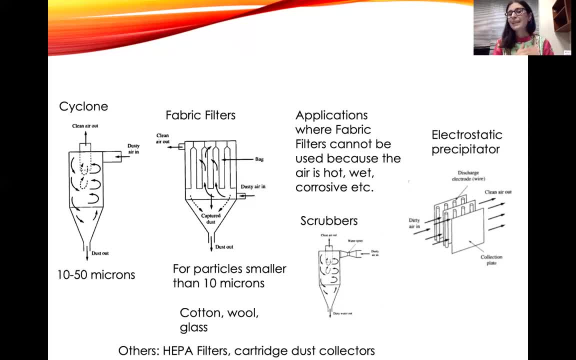 just dust right, so it can be something difficult as well. and when that happens, you introduce water. so there's the concept of wet scrubbers, where you introduce water, make it a part of the water and then treat it um and and that process is generally called. so basically, the water. 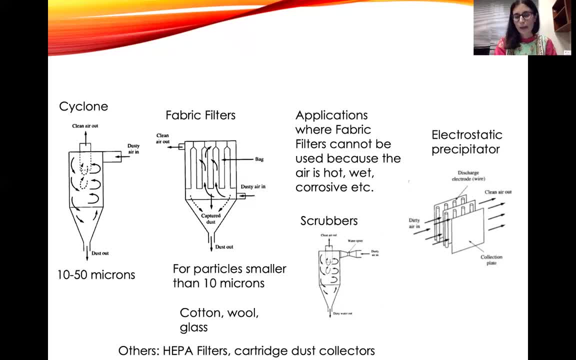 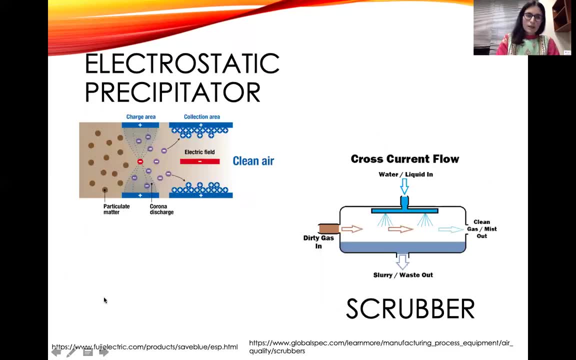 weighs it down and washes it and allows only clean water, clean air to go up, because air would just escape anyway. and different kind of cartridges and filters are used- um, let's not discuss it here- and uh. so so this is this. is it nadia? it's. 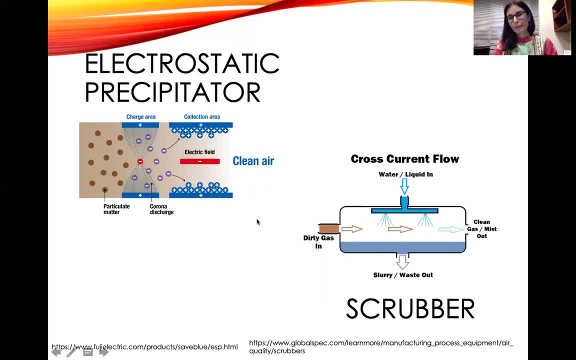 basically, you need to remember these two um, if, if i talk about it and not not like cram it, but just know the concept that what is happening, um, and why is an electric field being applied, uh, and how's that static charge being developed? and then how does a clean air come out and for 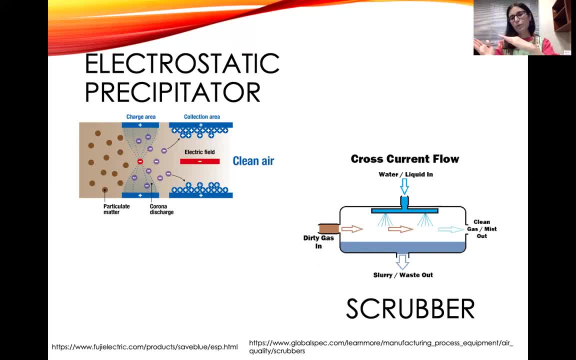 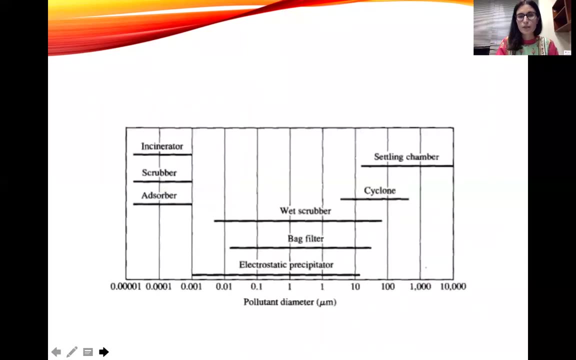 scrubbers as well. like this is a cross current, it could be a co-current as well, so just know that these are very easy, easy, scientific ways that have been used in bigger gadgets to solve bigger problems of air and environment. and and, for example, if i say that we have to take care of lahore's, 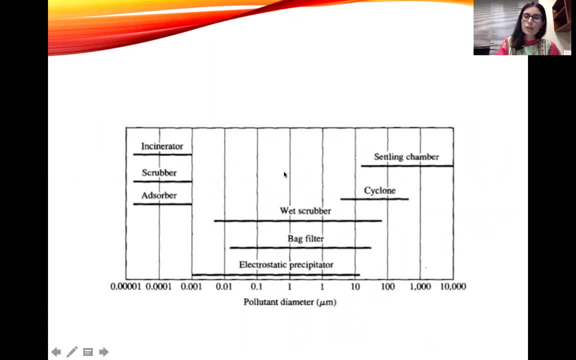 we know that the particulate matter 2.5 is really high. so, depending on what the particle size is, if i tell you what should we install at the industries today, and you see, settling chamber, that won't be the answer, because we have a very high particulate matter of 2.5 micro grams per meter cube. so maybe 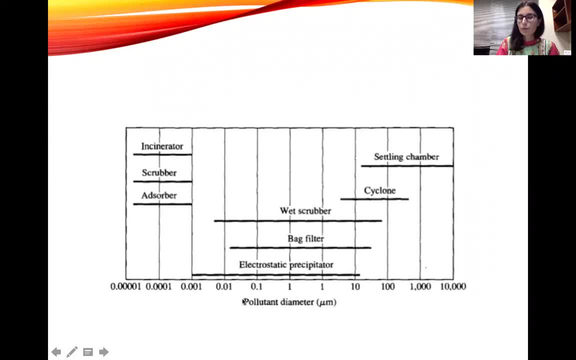 like in terms of microns you need to think about. you know, maybe stay in this range to make sure that the air in lahore is clean. so just for you to make those decisions based on what the size of the filtration process is. now let's jump to the gaseous pollutions. 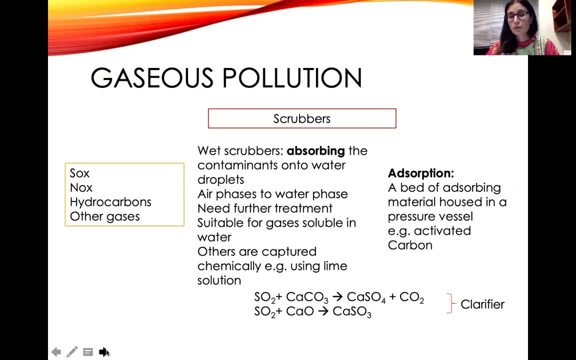 who can we quickly recall the gas solutions that we pollutants that we've already studied in the course? somebody else, manal, um, so there was a sulfur dioxide, and then uh, variants of um like, like noxes, nitrogen dioxide, um, i think, ammonium nitrate um, and then there was uh carbon, various. 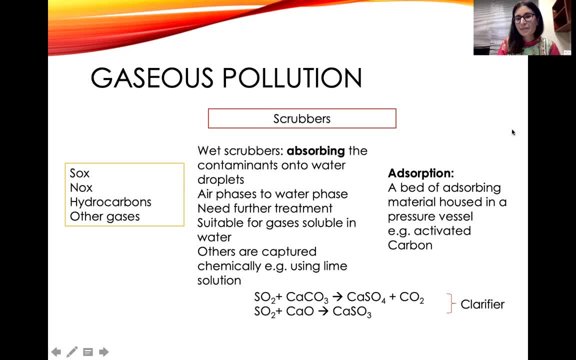 uh types of carbon, like carbon dioxide, carbon monoxide, um methane which were, which were greenhouse gases. um, i'm trying to think of the other ones. i think variations of, um phosphates of phosphorus, uh gas. um i'm trying to think of- i think that's it, i'm i'm not sure. 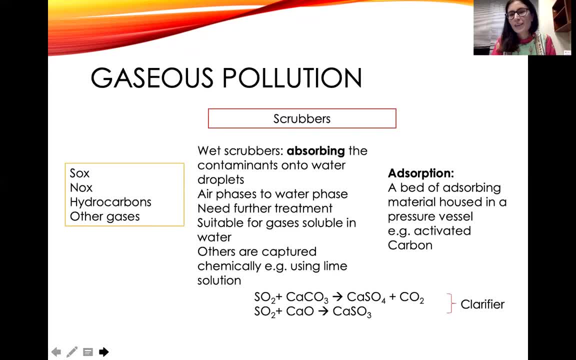 if i've missed anything, okay, okay, okay, i'll not. i'll not discuss what you've mentioned further, but basically we we talked about those um, classical air pollutants, yes, um, and that includes ozone and cfc and all all the rest um, and you know we can talk about what is being released. 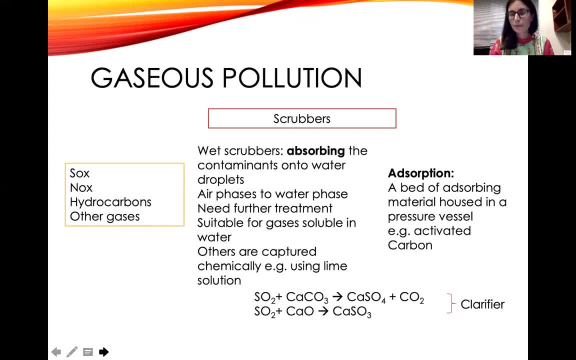 excessively from where and how and where it's impacting people or environments, but generally you categorize them into- you know socks, there's not says hydrocarbons. and then other gases could include ozone, um, etc. that are released or are a byproduct of industrial processes. the same 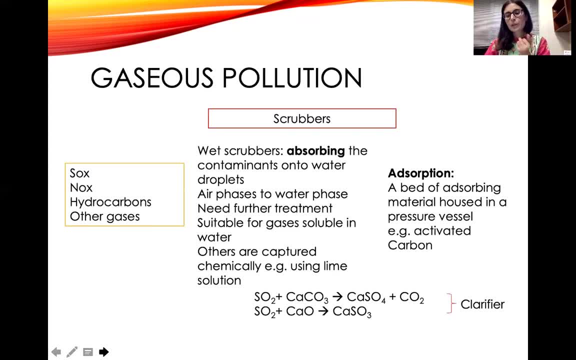 equipments could be applied here as well. it's just a different principle and, uh, maybe the chemists should finally speak up if they want to. uh, so basically, what you're trying to do is now the you know in in the particulate matter capturing process. we were 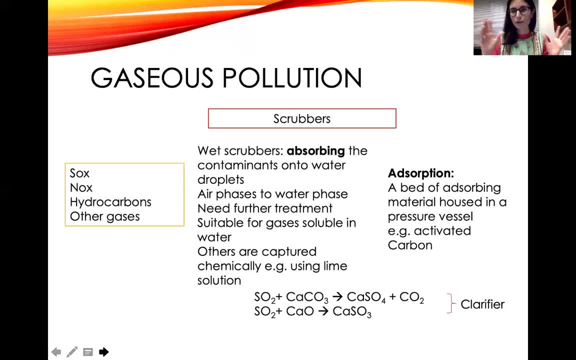 just allowing the gases to pass through, because we were saying it's it's oxygen and nitrogen, whatever it's not harmful. but now we know that it contains these gases and we have to capture these gases as well, which means that you have to stop the air. but but you can't really stop the air, right? so how do? 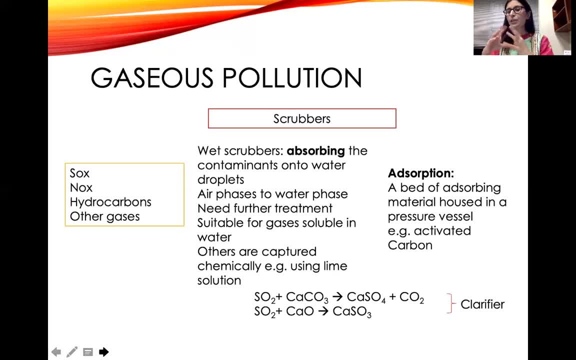 you stop these particular gaseous pollutants by dissolving them in water. if they are soluble in water- not all of them might be soluble in water, so then, of course, what happens is, perhaps these covers would have some water, they would capture these and then they would react with something. 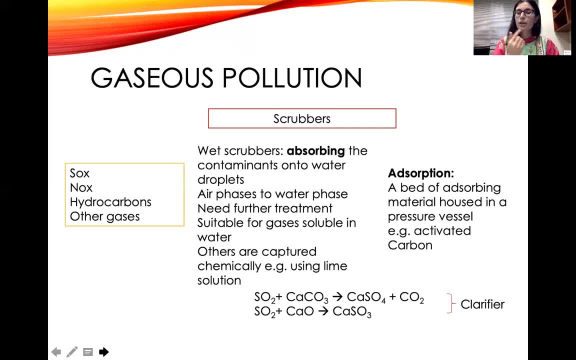 or maybe you will. um, i think, as someone writing you mentioned, the walls would have certain chemicals. there would be a bed, so maybe these scrubbers would have a packed bed where peat or compost or activated carbon- which is again carbon- would be used to absorb these. just keep it on its surface, not allow it to escape with the air. 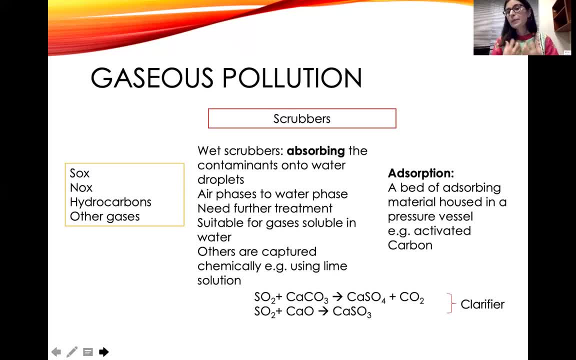 so it could either absorb it. absorb it so, for example, take it in, like dissolve it in water and then treat it, or it could simply absorb it, that is, it to attach to the surface of that bed and then only allow for clean air to pass through. and again, these are not very difficult scientific principles, you just use their characteristics. 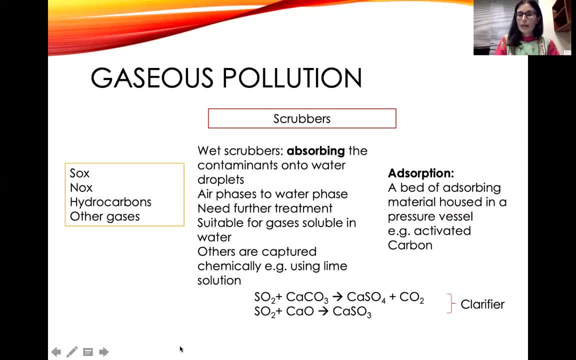 and these are all very established, well-established concepts as well. but uh, i forgot who had mentioned how sulfur is taken care of. but you know sulfur, for sulfur lime is is an absorbent um it. it reacts with it to make calcium sulfate, which is less polluting. but there's 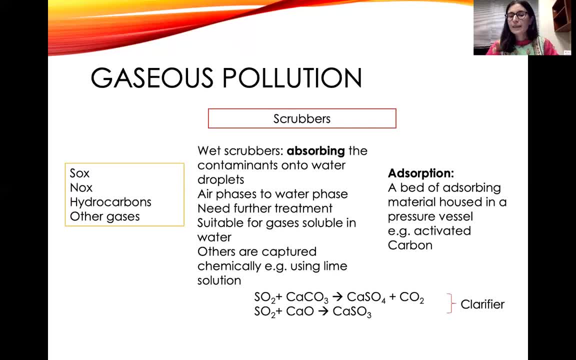 a lot of other different ways of doing that with with the other solutions. so we- yeah, i think these are low, but i'll just- i'll just add a little detail. i think this is a very common result, but of which we also have a particular example. so, as we think about it, um, copper is, uh, a very 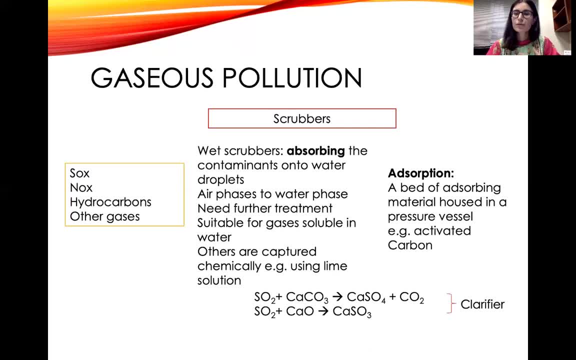 common process in the environment, because copper is a very important liquid and we often use copper for other things, uh, like solar panels at our own sites and other plants, and we have two other systems in our own system which is the backbone of the carbon dioxide system, and the carbon dioxide is the greenhouse gas. so even if you're reducing one pollutant- which perhaps could be could be difficult- you're still creating another pollutant, but the good thing is that carbon dioxide is easy to capture with plants. i'll let you go ahead and go ahead and start with the next question. 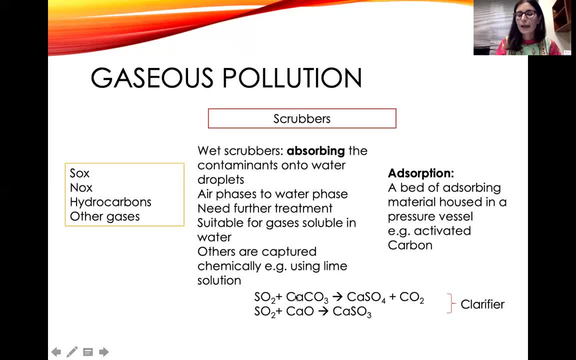 So if we plant more, then perhaps we could capture this, And this is a more dangerous one compared to this. So I think by creating the carbon sinks, having those agricultural practices that we discussed in the course, maybe we can take care of some of these pollutants. 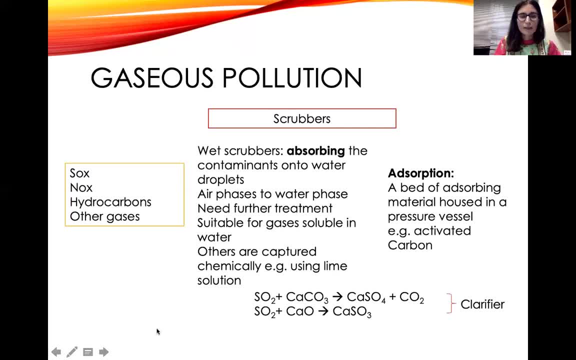 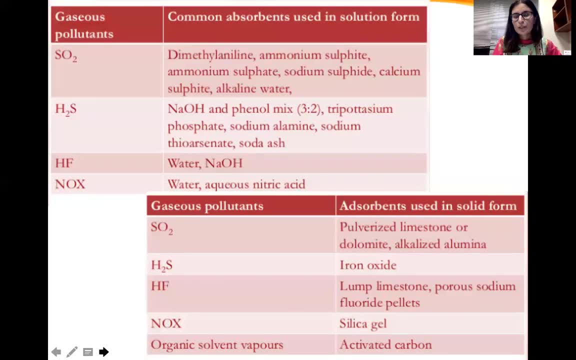 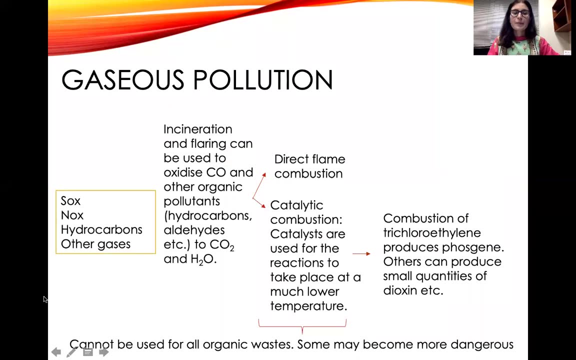 Any question here, guys, Because I can't hear you And it confuses me whether you're understanding what I'm saying. So this particular slide is for the chemists. I wouldn't get into details here because I think you're already scared. 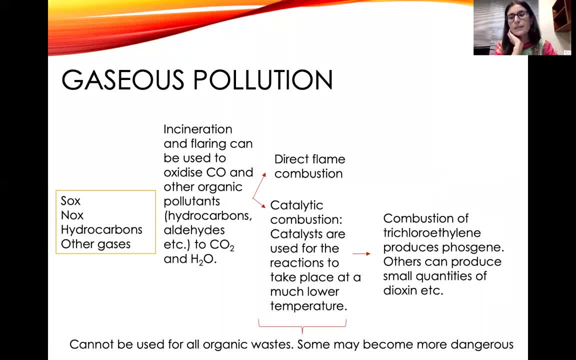 Also, we've discussed incineration, So someone has to remember what incineration is and tell me what it is. Anybody else? Azhan, where are you uins? OK, Iman, have you spoken? Iman can speak. 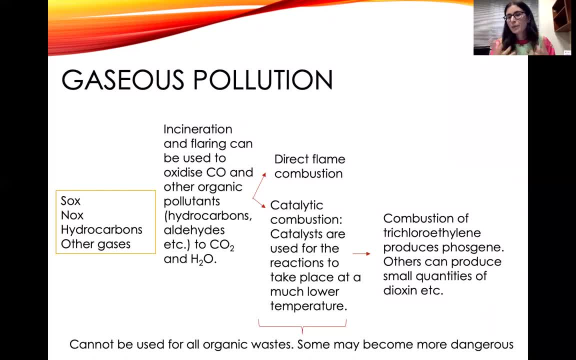 Yeah, It's when you burn waste material. Yeah, So we basically burn waste material And, like I said, in the process of combustion, CO2 still released wood. wood, which is biomass, is also cellulose, and cellulose is basically a hydrocarbon, which means 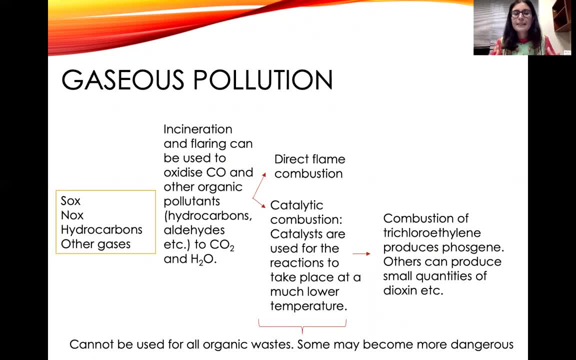 it contains carbon, hydrogen and oxygen. so when i say that there are various hydrocarbons like, i'm giving you a very easy from your day-to-day life example. but these hydrocarbons could vary, you know, and they could be more difficult hydrocarbons and, and those hydrocarbons are: 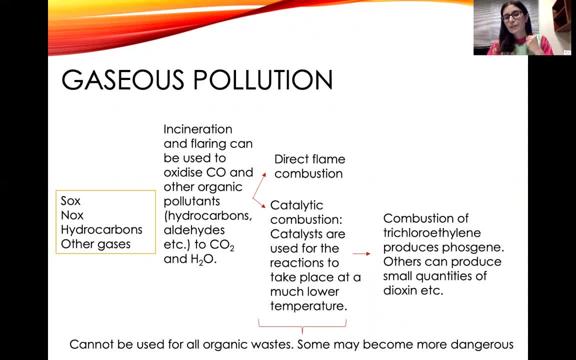 basically just put in into these incinerators at a very high temperature and pressure, we burn them, and when we burn them we release not just carbon dioxide and water, but a few other flue gases as well. uh, but, but you know it's. it's still better than, i think, sending all of that waste into. 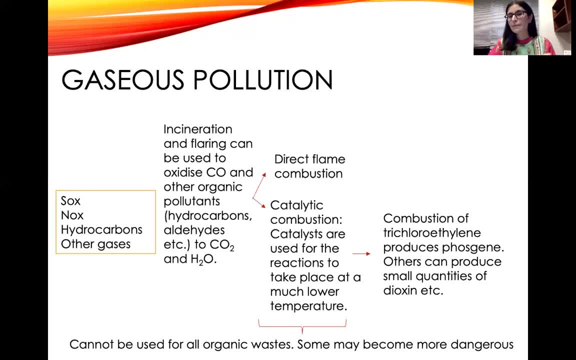 landfills and then all of those gases into the air. it's still better than than that and of course, you can use direct flame combustion, so what you see at the end of the landfill. so when a landfill is closed, there's always a chimney or a pipe that has flame. that flame is basically the biogas that's being released from the land, from. 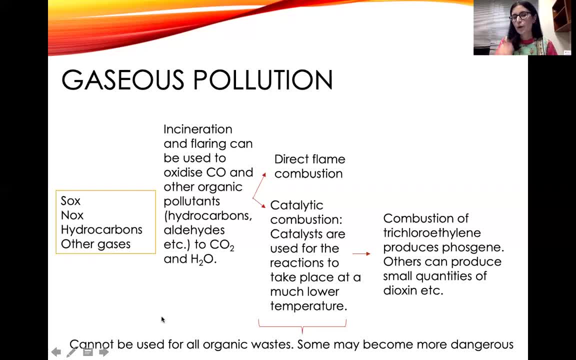 inside the landfill, so that would be a direct flame combustion. you're just burning it, but you could do the same in the incinerator as well, and sometimes it's catalytic combustion. yes, azam, do you have? you want to say something? yes, but yes, ma'am, i just want to add something. go ahead. 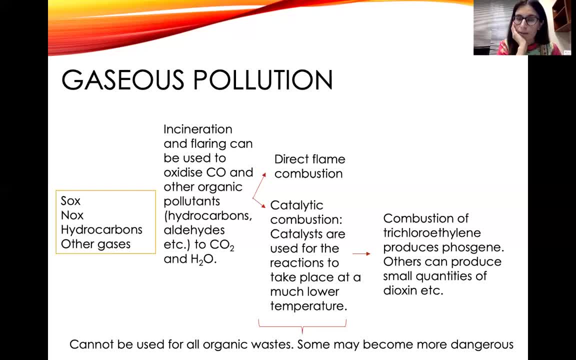 thank you. so the thing is, you are mentioning greenhouse gases or stuff like that, but i just want to comment that you didn't mention, uh, water vapors uh, because i feel like most of the students don't consider water vapors as a greenhouse gases. so we will uh talk about. 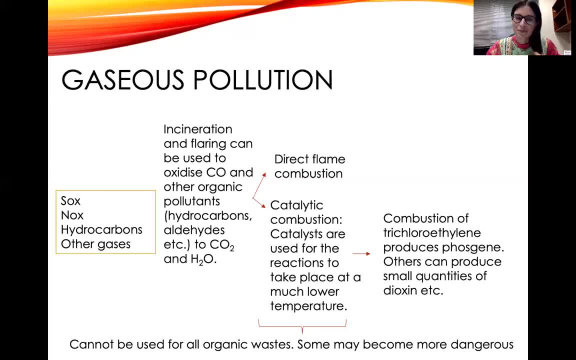 this as well. uh, like, how to incorporate this because, uh, you, you know that uh water vapors are also i are active and they are absorb uh radiation and causing uh global warming. so just you mentioned it was systematic. i think it's too obvious. yeah, i think we systematically do that and then, like, like you mentioned, carbon. 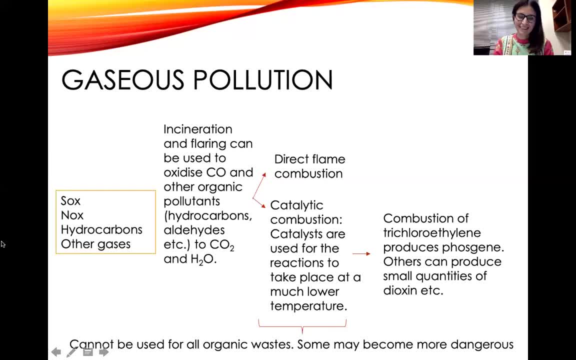 dioxide, methane and other gases, but i feel like uh, water is also a major contributor. it is, it is, and i think a lot of the counter argument on these gases is the fact that it's actually, it's actually also does absorb water, but that's its ability, right we? we say the same thing for ocean. we say: 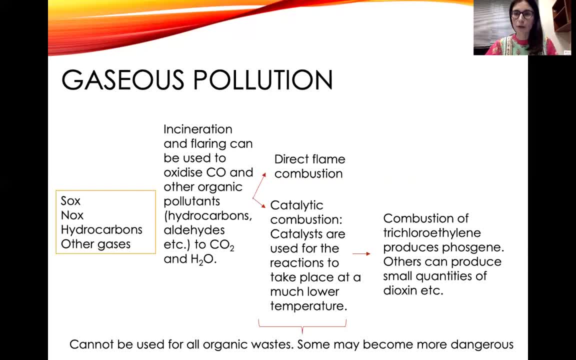 it's, it absorbs the heat releases for all all water bodies that are present on earth. they capture, store heat and then release it slowly at night. um, similarly, the water vapors that are present in the air act as a greenhouse gas, because that vapor is now, you know. so steam is basically. 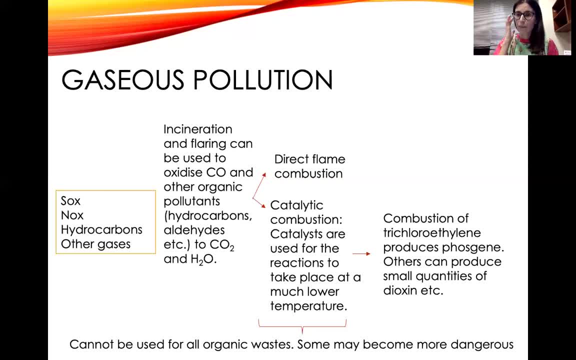 so, like we say, water has three forms, right, so that's the gaseous form, um or um. let's say: if it's just in the. this is the gaseous form um or um. let's say: if it's just in the, if it's just in the. 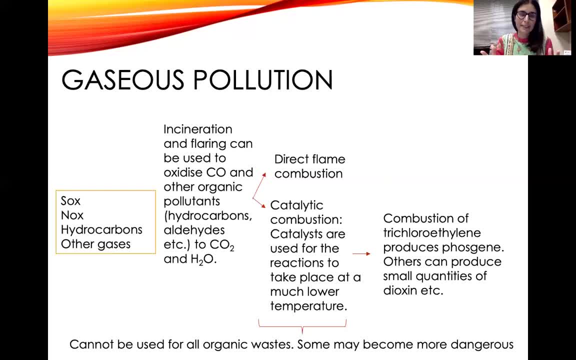 dense form in the air, it would absorb water because that's its ability. we we studied the characteristics of water. that's its ability and I'm not going to deny this. I know a lot of science proves that it's so much more. it has the ability to absorb more heat as well, I think. I generally do not want to sway. 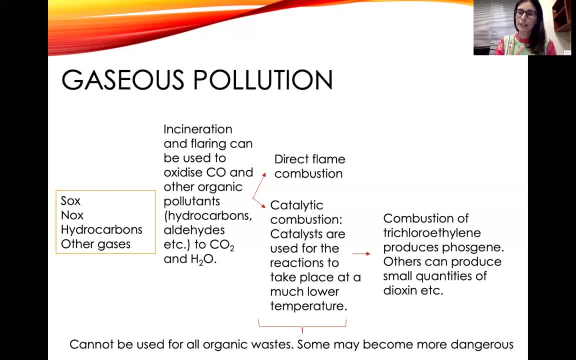 away from the discussion of the pollutants that we are actually putting in the air, because the water vapors in the air are a part of natural water cycle and and that was natural water cycle has, unless we are human activities and increasing the water vapors, which in some case we do- for example, an airplane- 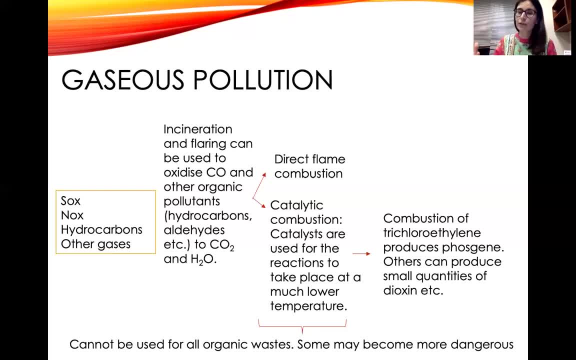 could release a lot of water vapors and they could also increase warming of the atmosphere. but I think because, a- it's a part of the natural process, so the natural water cycle process, and B- it doesn't have any secondary effects. if someone tells me that you know, forget. 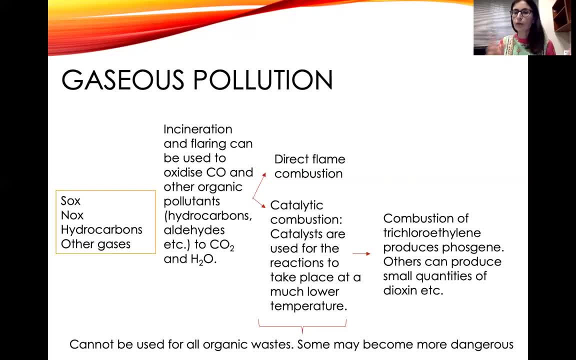 or forget anything: water, hat water- is equally a greenhouse gas or a planet warming material in the air. I don't think that comparison is fair because, yes, it can absorb all that heat, but it's secondary impacts on the on the planet are really really minute. so I don't think that comparison is fair, but yes, I. 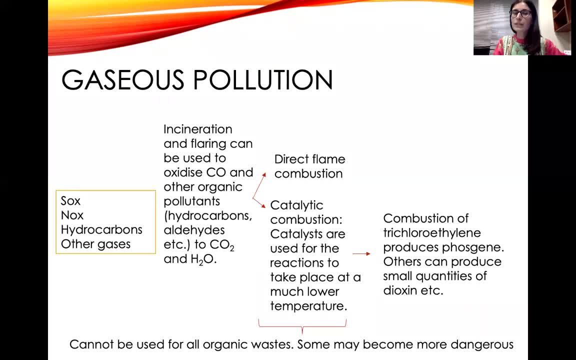 haven't mentioned it anywhere, so thank you for bringing this up. as on water in the atmosphere on the planet, anywhere in the world, the earth in reality has the ability to absorb water, so right. so when it is solid, how it's compact, when it's liquid and then when you heat it up, how it. 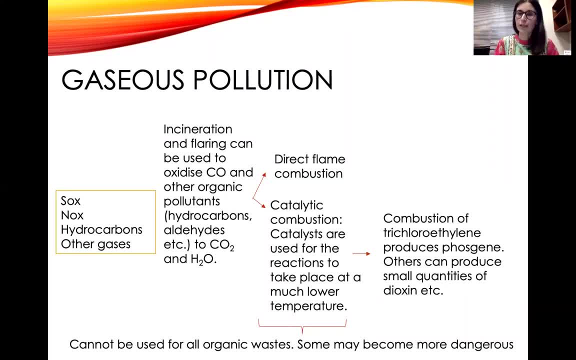 keeps absorbing heat until it releases those wafers into the atmosphere or turns into the gaseous form and it can have. all of those forms are something that I think everybody knows. so I didn't really focus on that, but I was hiding that information on purpose. but since you've brought it up, yes, water too is. 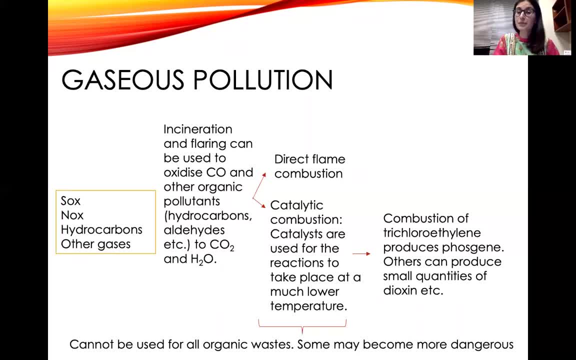 warming our planet and a lot of counter climate change discussions be known, but that's my reason to not bring it up. so the purpose of like sharing this or like bringing this up is to make is to accept the fact that most of these two students that we have in the class are from non science like on. so it is they should. 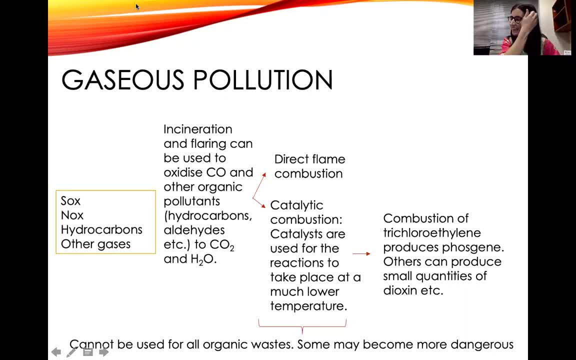 know that. this fact that water vapor is also a major contributor- yeah, but they aren't an air. They are a contributor to DHG, they are a contributor to warming the planet, but they are not pollutant. Yeah, obviously they are not air pollutant, but they are causing global warming as well. 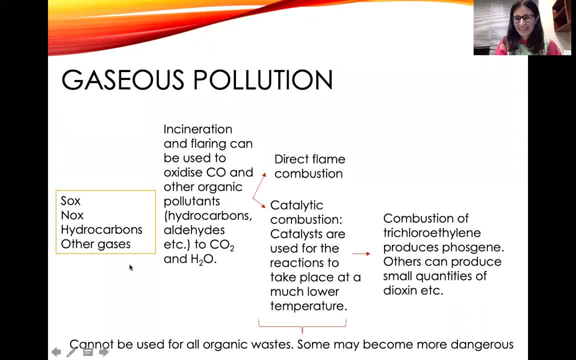 They are. I'm not going to disagree with you. Okay, but thanks for bringing this up, because I think I have never mentioned it in the class. And then, of course, let's then not talk too much about the combustion process. but we 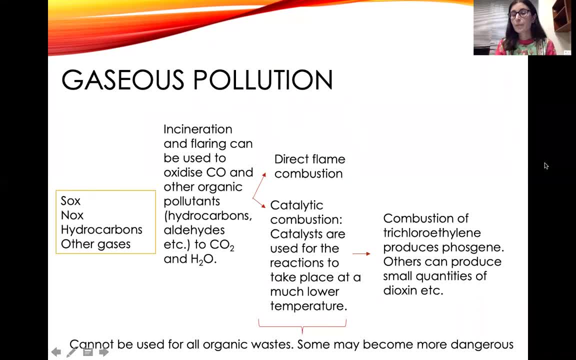 basically in the incinerator, using certain factors, burning things up, And the process of burning is not always good because sometimes, like we said, organic waste can be burnt, but not everything that's burnt and not all the products that are being produced. 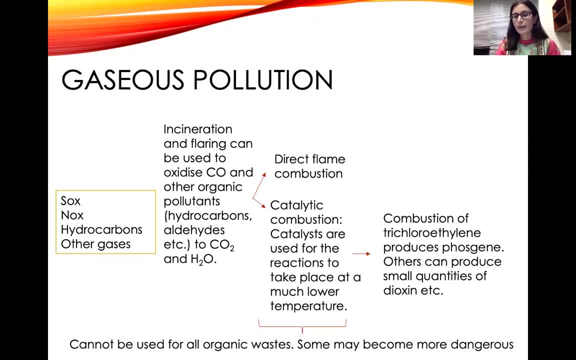 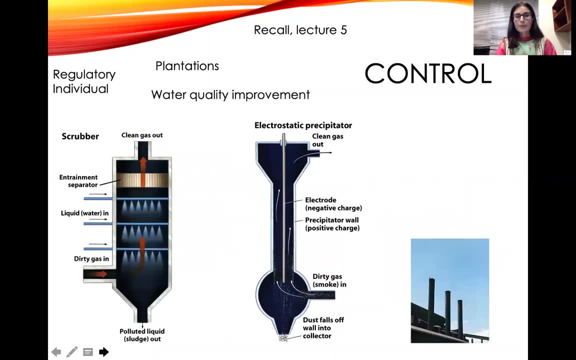 are good for the planet. Sometimes the by-product is more dangerous And I think I've given an example of phosphagen or something on the side which you can read. This is a lecture that I wanted to. I want you to recall lecture five, maybe you can. 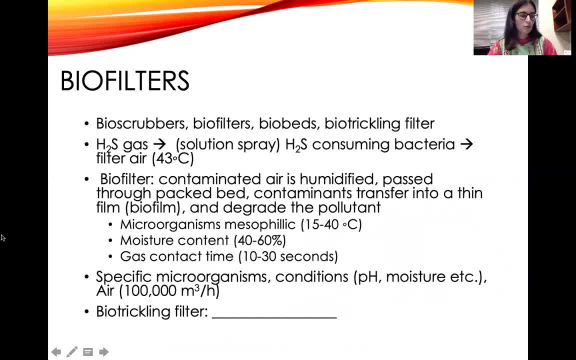 think about it again. So, basically, this will now bring me to the point on biofiltration process, And I think this is the most important, because I think all the other things are more chemical engineering, or maybe mechanical and chemical engineering in combination, to keep our environment. 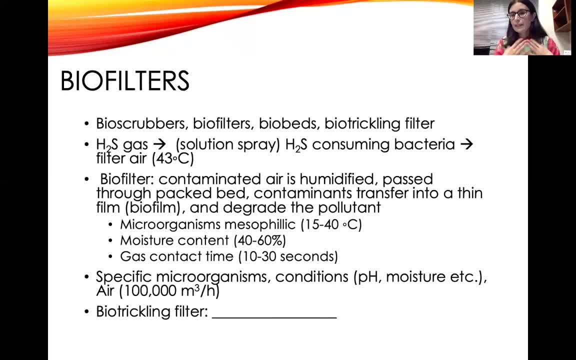 clean. But here it's sort of that interface that asks us: Okay, Okay, So this is what environmentalists like, right, Where you're not only thinking design and you're not only thinking physical filtration. So not only physical treatment, not only chemical treatment, but also biological treatment. 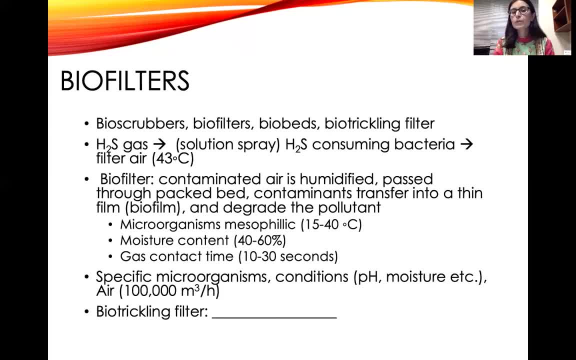 So thinking about mimicking nature and using those microorganisms or fungi or plants or trees that can do the job for you as well, But in moderation, like I like to use the word moderation everywhere. So basically what you would do, for example, is in the same scrubber. 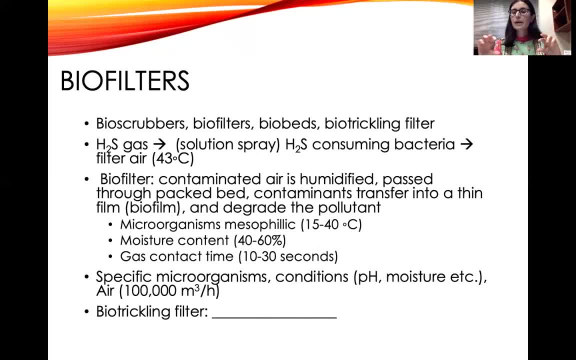 You could have in the packed medium peat compost that you produce at home. that could be your bed where you grow microorganisms, and those microorganisms would have the ability to degrade, let's say methane, sulfur dioxide, H2S gas, et cetera. 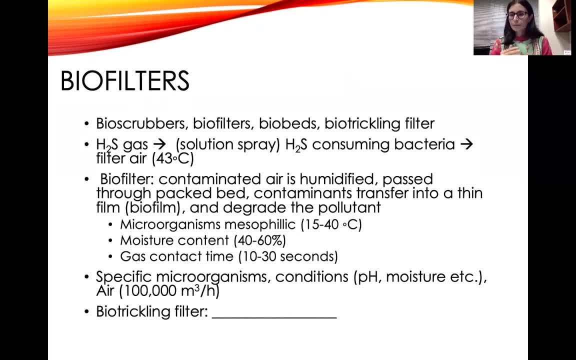 So that's how it's designed, but it's not as easy as you would think. There are a lot of experiments that have to go in to bring it from the environment to the lab, To kind of sometimes genetically engineer it or to know the exact conditions right. 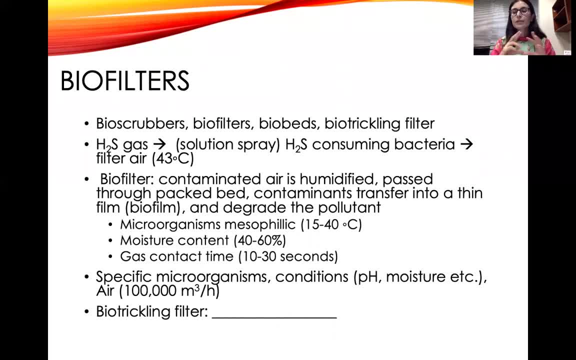 Because sometimes isolating them from the environment is also not easy. Then to find the right conditions, the optimum conditions for the bacteria to thrive, grow continuously, grow to get rid of that pollutant is a principle that biologists have to develop alongside that material or design to ensure that the environment remains clean. 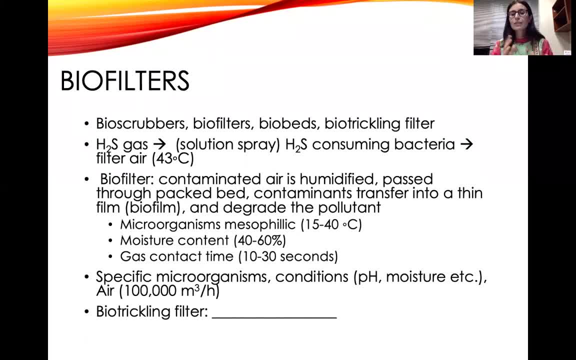 And when you have those conditions, I don't think it's difficult to establish a similar setup elsewhere, And of course you would. you know, if it's aerobic bacteria, it would need oxygen. If it's anaerobic bacteria, it would need no oxygen at all. 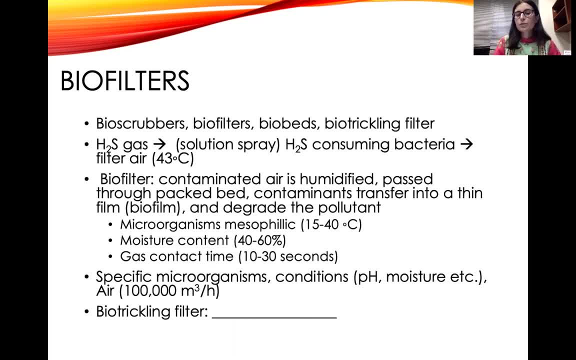 Then you would maintain the pH, the moisture, everything else that's important for whichever bacteria you were thinking about. Generally, in treating pollutants specifically for industrial wastewater and industrial air, the word biofilm comes a lot, And biofilm is a very important word. 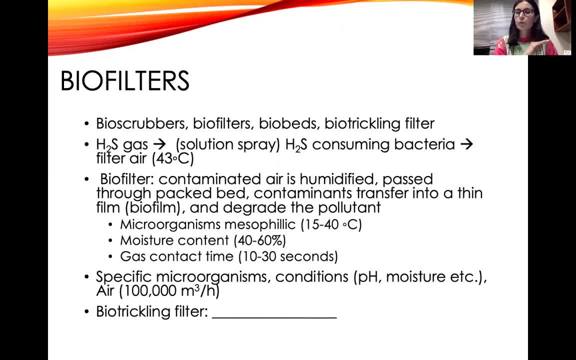 It's a very important word. It's a very important word. It's a very important word. And biofilm is basically the thin film or the thin layer of bacteria or fungi or anything else that will be formed on a surface. And I think I mentioned it before as well. there's an interesting equation where bacterias 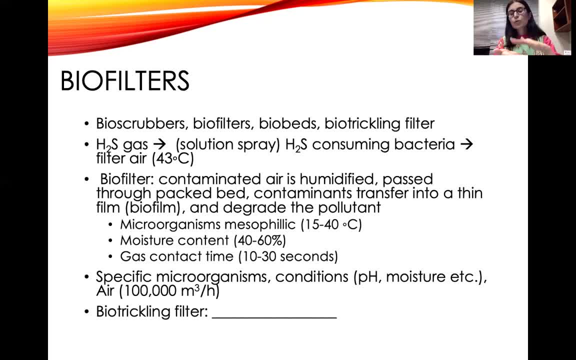 grow, and then you know they grow on the surface. Then, on top of that, another layer of bacteria grows. on top of that, another layer of bacteria grows And what happens is that you have this nice aerobic, anaerobic population growing in to. 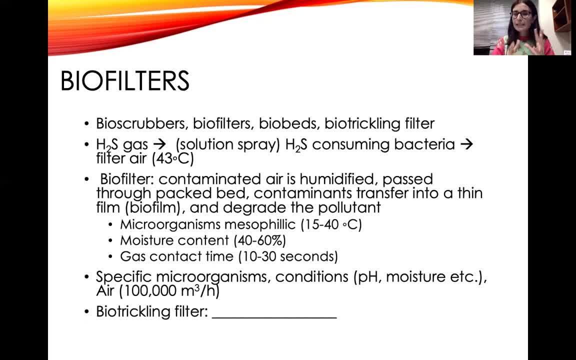 take care of the pollutants, So they're simultaneously, They're coexisting- to get rid of the pollutants that we have produced, where the ones that are inside have matured and are growing without oxygen and light and treating one kind of pollutant And the ones that are on the surface are thriving, growing fast. 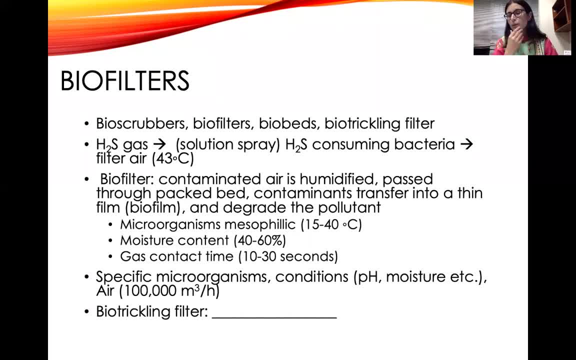 The ones that are inside are growing slow, And then they're trying to treat a particular pollutant in the environment for us. If you want me to talk more about it, I can talk more about it. If you want me to jump, you know. so I've given some conditions, some examples here. 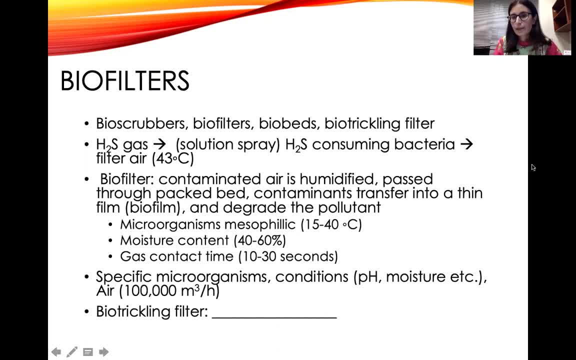 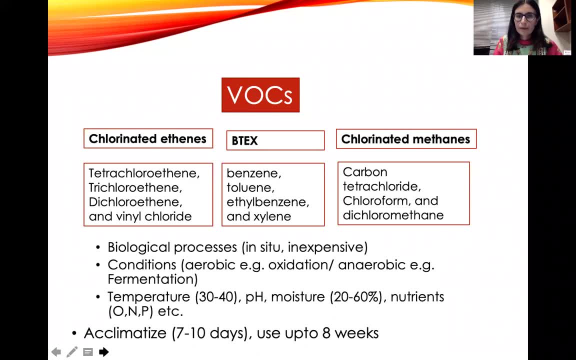 For you to follow as well. So if anybody has a comment, any example, any question, you are more than welcome to ask. No, Okay, So I think now I have another question for the chemical people which is I've been using 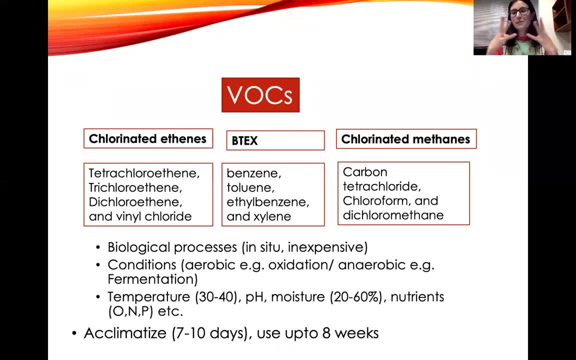 genetic terms And, to be honest, I should be, Should have expanded a little bit, Okay. So, for example, because even these times I think you didn't familiarize yourself a lot with yourself. So, for example, volatile organic carbons is a set of elements. 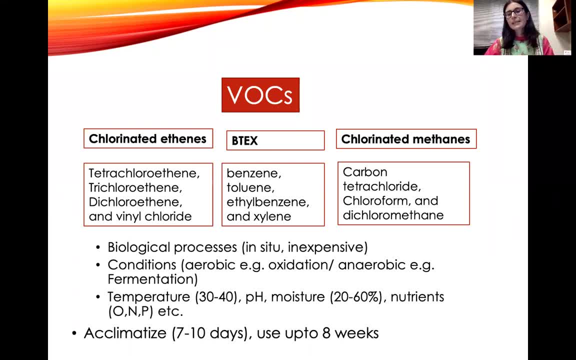 And they are. even those are categorized in different categories. So when I say we are using biofilter or a bioscrubber to get rid of volatile organic compounds from the air of an industry, it basically means you know one of them. 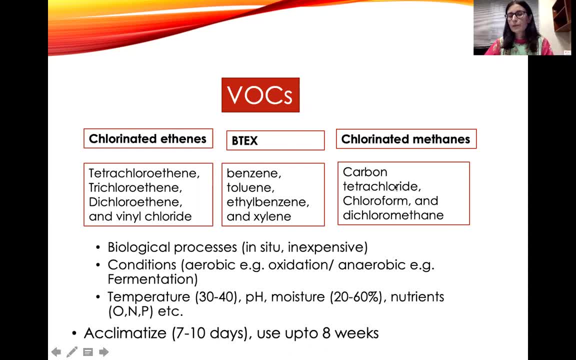 Okay, Okay. So you have these Many chemicals, or maybe few of these Chemicals, the the entire list, And of course they've categorized it. You probably hear benzene, ethyl benzene, et cetera, a lot. 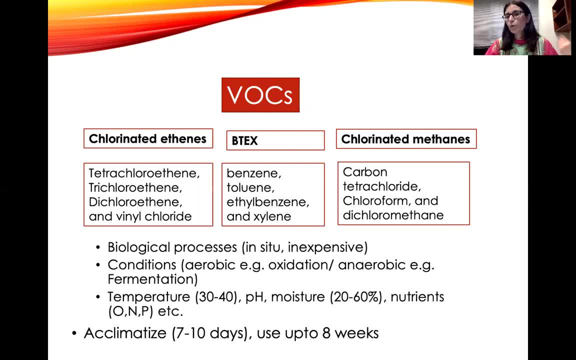 And and then, and then the other side, chloroform, which which are used in the labs and stuff. But why is everybody so quiet? But yeah. so basically what I wanted to do here is make that combination between biofiltre. 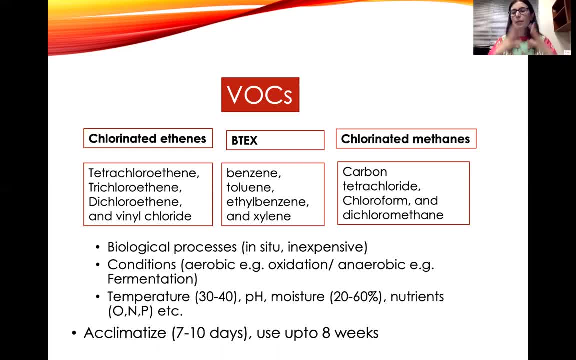 or that technology where microorganisms are used and bringing in a complex- Oh yeah, complex- set of chemicals. So let's say we're talking about volatile organic compounds and we are saying that these could be degraded by microorganisms. Now why do we want to? 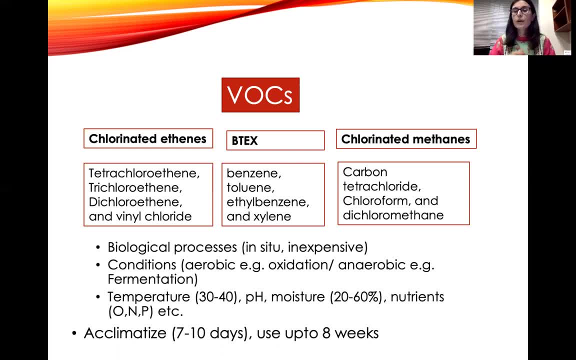 rely on biological processes Because it can be done in situ. In situ means wherever the pollutant is right, So on source, at home, And then it's inexpensive. Like I said, you don't pay a bacteria for doing the job, You just make the conditions right and they do. 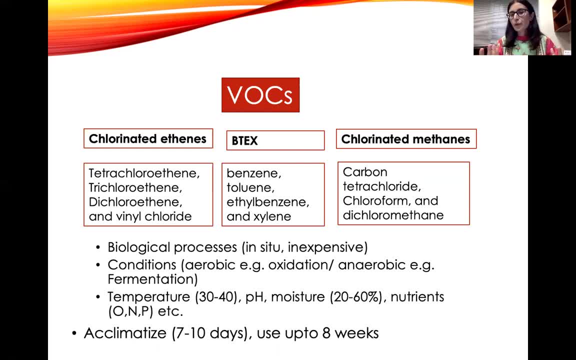 it. You only need to provide the right conditions for them And you need to give bacteria the time, or fungi the time, to acclimatize into that environment and then put it in that particular place. So, for example, when you hear a solution of bacteria was sprayed on wastewater or sprayed 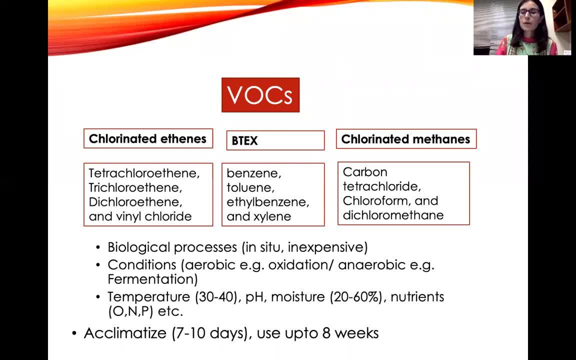 on the soil to take care of something. it would probably have been acclimatized, and then just it's growing, it's thriving, And then you put it in a certain environment where there's pollutant and it takes care of it, And if everything else goes well, like if the nutrients and all the other conditions 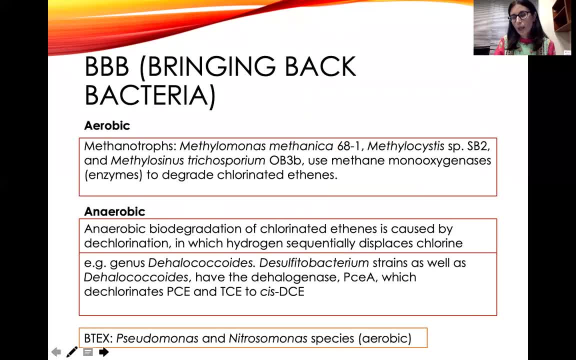 are there. it should be able to grow very well And should I talk? So I just want to credit the bacteria, because I always keep saying bacteria, bacteria and I never really put a name. Well, I do sometimes, but you know, there there can be all kinds of bacteria. 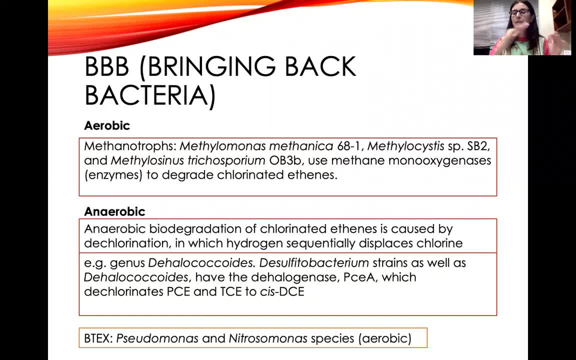 that would treat these volatile organic compounds for you, Sometimes in certain processes. Again, the names would be easy for biologists and scientists, but you can know that these aerobic and anaerobic compounds are basically hitting those chlorines away from these volatile organic carbons and replacing that with hydrogen and rendering them less toxic for the environment. 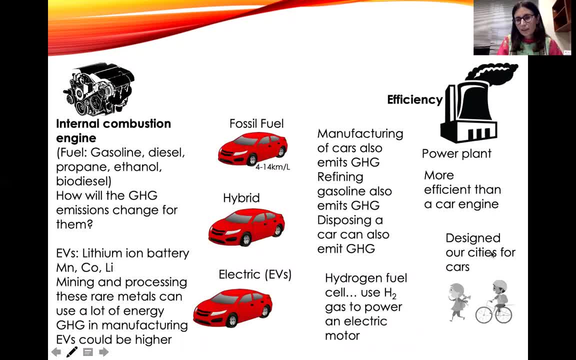 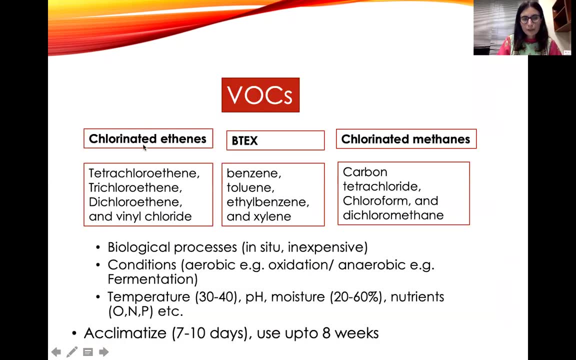 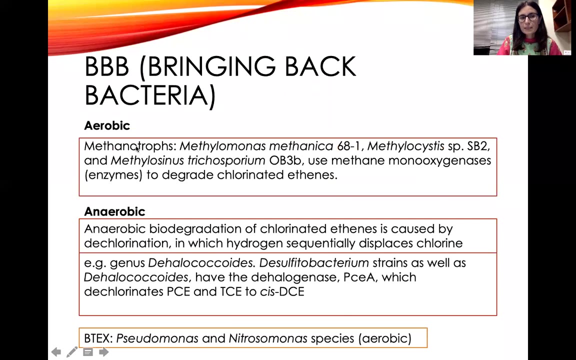 Any questions? Yes, Daniel, Okay, Which volatile compounds were you just referring to in the last slide? In the last slide, I was referring to the first group, So I just picked a few of these And let's say so, I said chlorinated ethines, right, And I was saying that basically these. 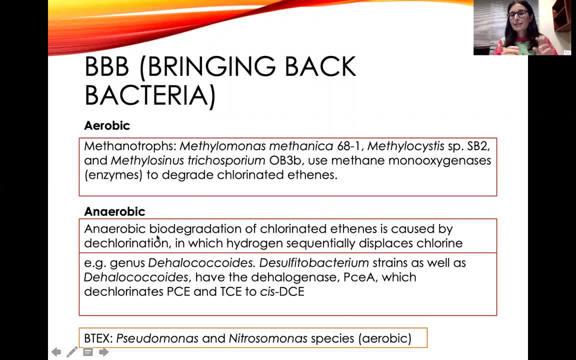 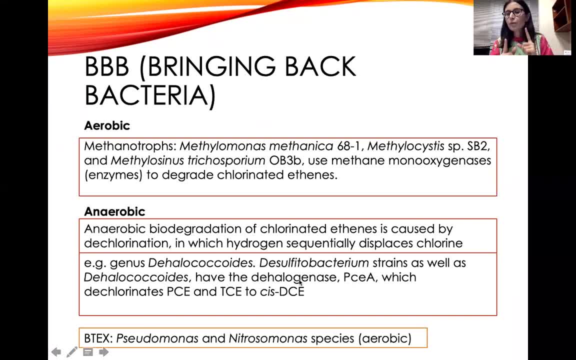 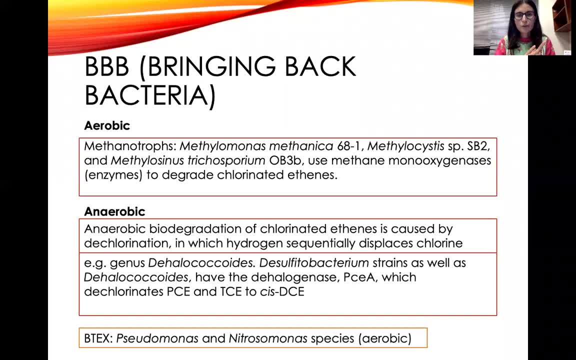 it for them And I think- right, They mentioned it somewhere so I just didn't want to highlight it- but a particular bacteria which has the right gene to to do that job would do it in the right environment, when, when it's given that that job. So yeah for those chlorinated. 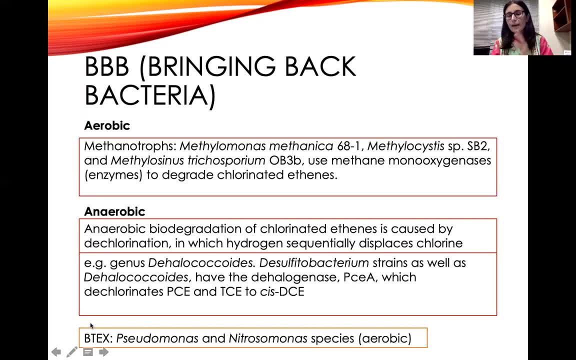 ethines, and then for BTECs, I think, I repeat it again, my my personal favorite bacteria, pseudomonas. it does the job everywhere. So yeah, in general- oh yes, I agree with you- Great. So for BTECs, I think Pseudomonas aeruginosa, Putida and Nitrosomonas species have been 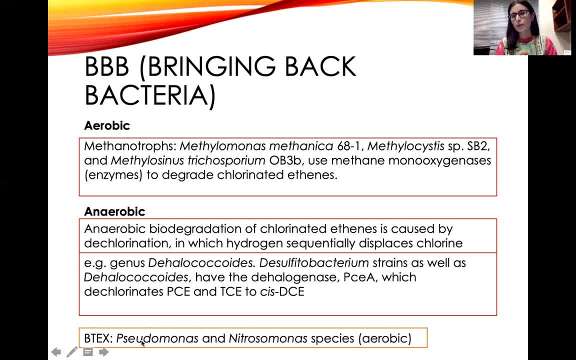 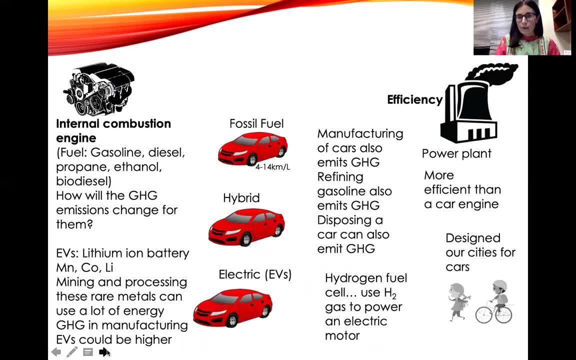 very effective in taking care of them in the environment and they're quite well known. But others, like Bacillus, etc. also do their job and they're easily found in the environment as well. Does that answer the question, Daniel? Yes, ma'am, thank you. 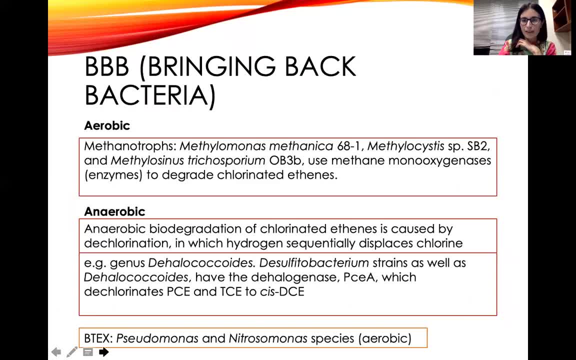 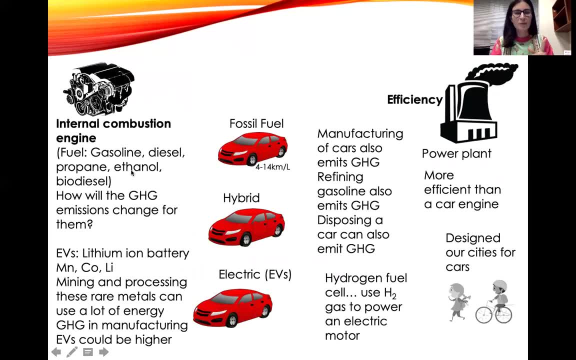 Okay Now is Hanan here today? Is Hanan here today? No, he isn't, because he's submitted an assignment on electronic electric vehicles, And so we have again discussed this. but I'm only putting it here for you to know that. 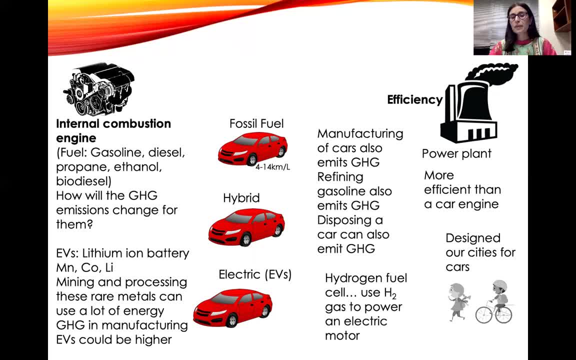 when you look at them from outside, they will all be the same, So some of them have combustion engines, catalytic converters converting the fuel Driving your cars, or hybrid that contain both the electric battery and the fuel, or the electric vehicles, and all they contain is the battery, which could be recharged. 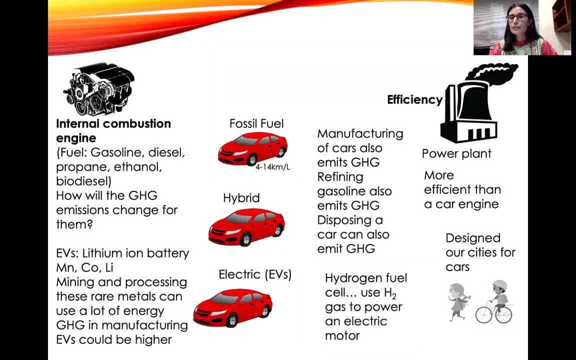 In terms of environment. I think what we haven't really discussed is the fact that a car and its manufacturing process is very GHG emission intensive as well, And oftentimes people who disagree with the rise of electric vehicles are not going to be using this card saying that the manufacturing process is also GHG emission intensive. 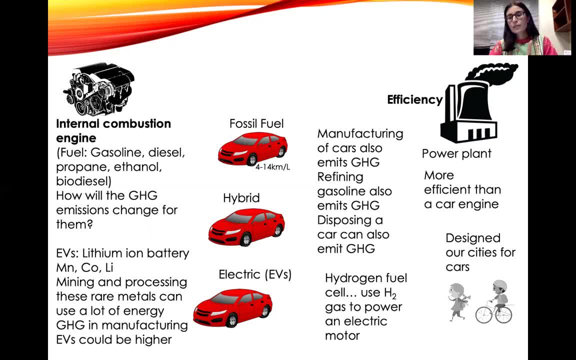 But I think- and then there is another narrative, and that narrative is the batteries use, which are the lithium ion batteries- They also use very rare elements such as cobalt. Cobalt is a rare earth element, right? And so if you're extracting them and it's already rare, then how do we make sure that? 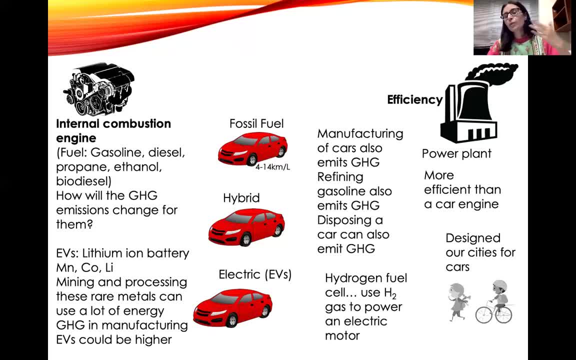 if we want to increase their numbers in future or if we want to increase the supply by also increasing the demand, by creating education and awareness, then can we really extract that much from the environment. And of course these are all the debates, but a lot of researchers have proved that. 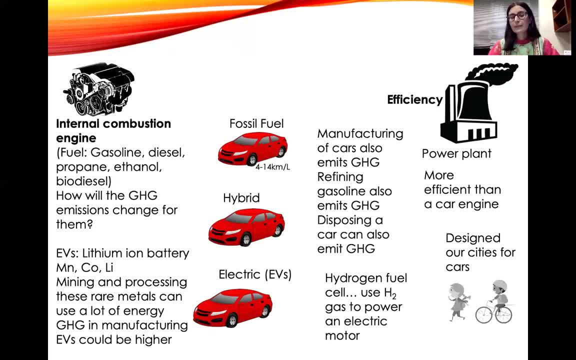 even if all of those taking them out of the earth, filtering them, using them in the batteries, the way of manufacturing the car produces GHG emission, in the longer run, electrical vehicles are still, or electric vehicles are still, better than the simple fossil fuel, or 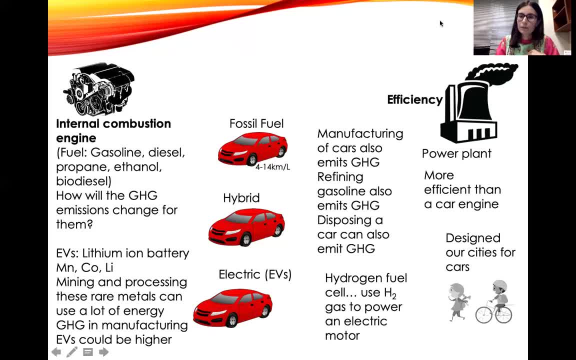 hybrid cars And, of course, the hybrid car is better than the fossil cars. Now, why should we worry so much about cars? Because, unfortunately, we have designed our cities for cars, And I think that's why, at some point, I wanted to discuss urbanization, but I will not, because 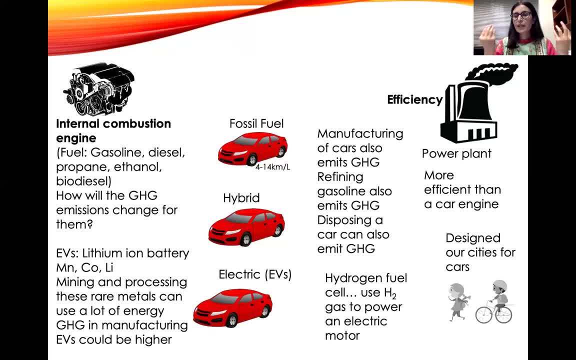 we don't have time, But this is what happens when you design your cities for cars. So now, no matter what happens, we have to have this demand for rising cars because public transport has its limitations. But there's also something that there's an interesting comparison, And, of course, the second thing, after fossil fuel use, would be to improve its efficiency. 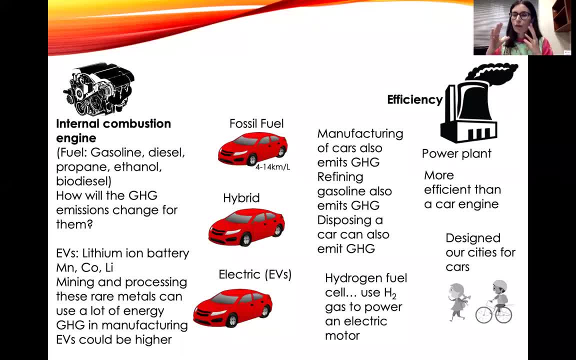 And a lot of people say that, even though a lot of fossil fuel is used in a power plant because it's used in a bigger setup and you can take care of it, and, on the other hand, the fossil fuel that's used in a car, that engine has a lot of waste, heat, etc. it's actually less efficient compared to that power plant. 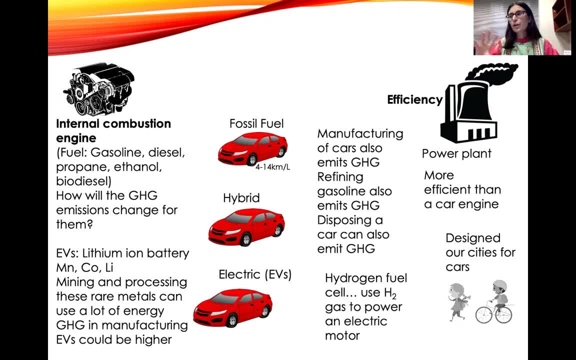 So if a lot of cars are put together and compared for use of fossil fuel, a car would be more inefficient than a power plant. So I think you know, as someone who knows what's going, where. you just need to think about these as well. 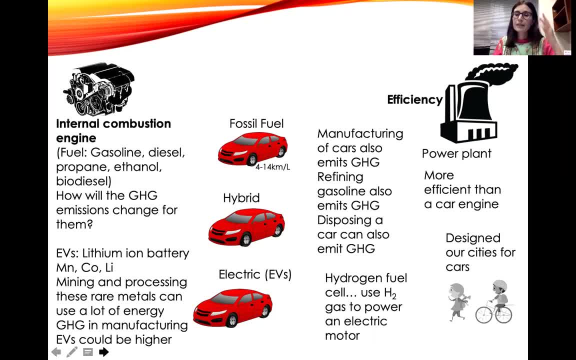 And of course there's the hydrogen-fueled car. It still is a long shot. even the electrical vehicles, even though they're being produced by Tesla and others, still need a much bigger market. And of course, hydrogen fuel cell, where hydrogen is used to power an electric car, needs to grow as well. 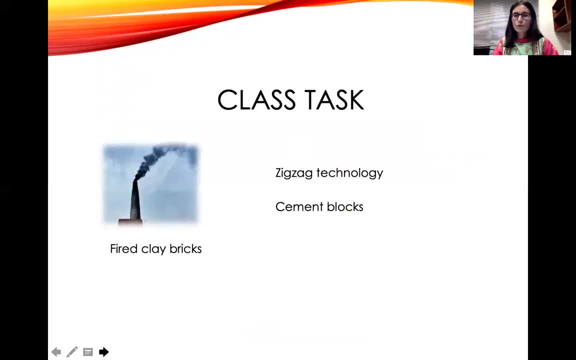 Okay, I wanted to discuss this, but maybe I can let that go. How much time do we have, Right? So you have five minutes. How many of you have seen a brick kiln? I haven't, so it was really hard for me to. 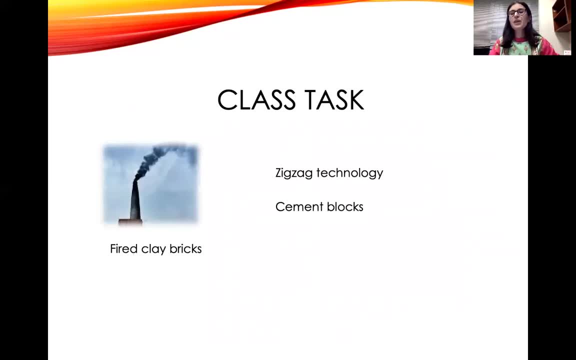 propose. Very good, Right, Okay. So basically, like I think Hasan said, we have to also look at the raw material and we also have to look at alternatives. Now we are saying that most of these fired clay bricks are a necessity. here, For example, in our area, we just use the cemented bricks. 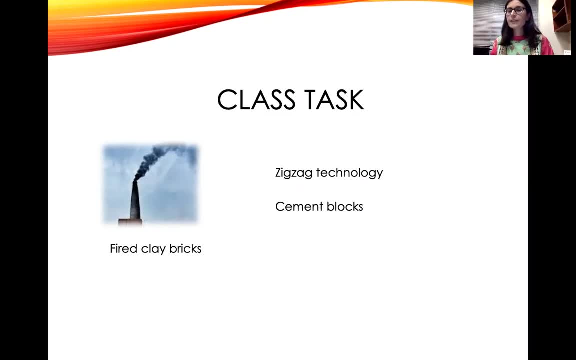 But apparently they are more expensive compared to these, and because these are cheap, that's why they're being used. I'm not sure about all the other comparisons, but that could be one alternative. But then the other alternative is to make these kilns efficient and sustainable, Right. 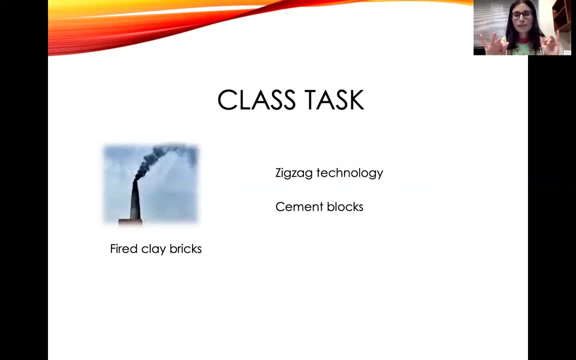 So I'm going to ask you to quickly use your such skills to find out what is zigzag technology and how is it improving the clay conduction or clay manufacturing? How's it rendering it clean, basically? So what is being used? Like the navel square, of course, something is coming in and zigzag. 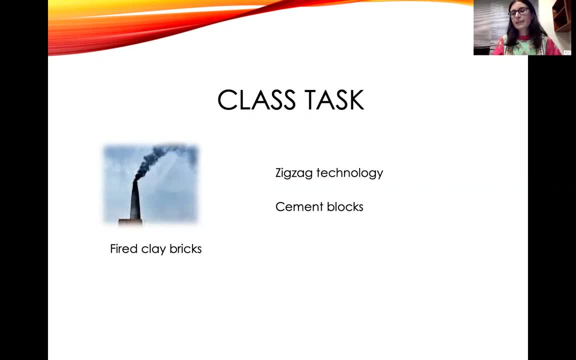 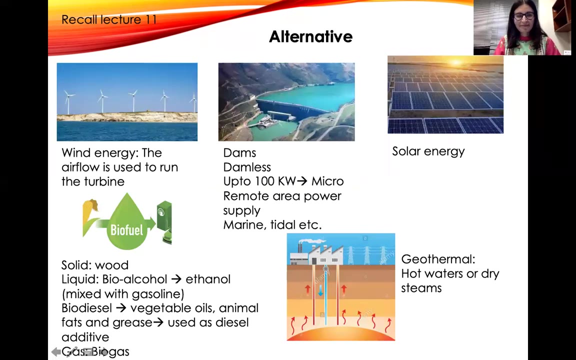 But then leaving the kiln. but how does that make the process better? do you want to do it at the end or do you want to do it now? now, okay, so you have, oh, i'm such a good time. okay, you have three to four minutes. 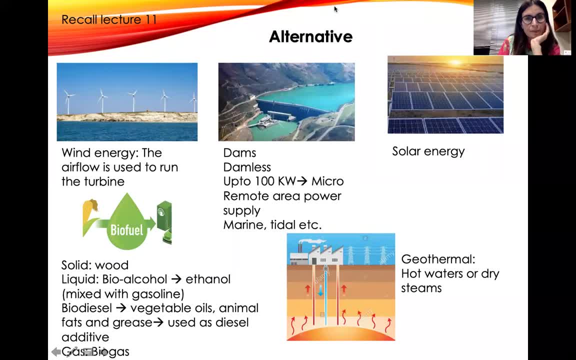 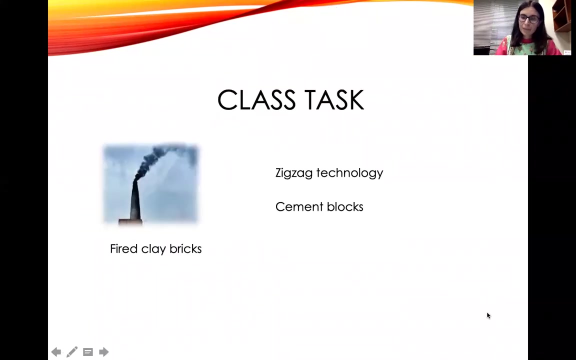 to search this. so if anybody knows anything about brickens- anyone who's visited it recently and can point out the you know what it, how does it operate, why is it good or not good- they can also kind of just talk about it. but if you want to talk about it, you can do it. at the end of the day, 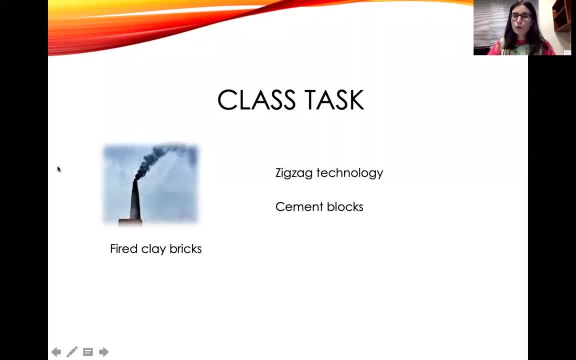 you can do it at the end of the day. now, did you want to talk? uh, no, no, i'm not sorry, it is from the earlier. okay, dean's raised his hand. i think. yes, ma'am, i have. i'm done with the research. so if you want me to talk about it, i can go ahead. 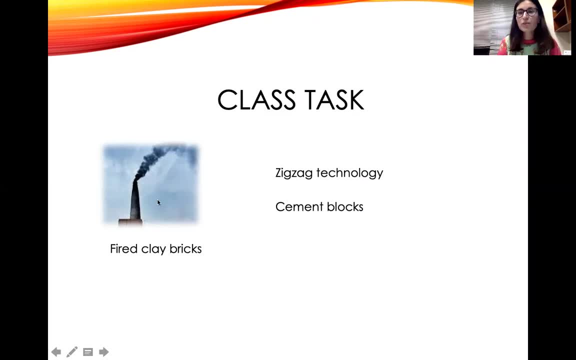 oh, can we get two minutes more please? you can. you can do it, the rest of you, but adin can talk. we also want to hear: i mean, why don't you type it and then why don't all of you who found the answers type it and i'll choose the best one. 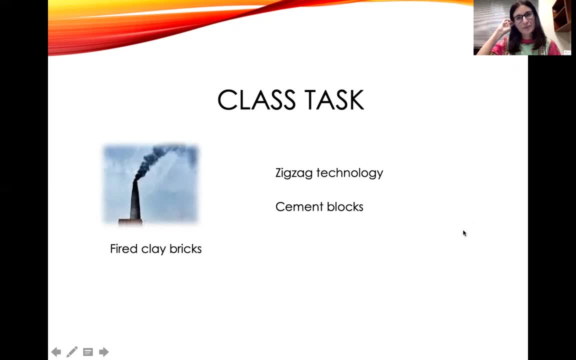 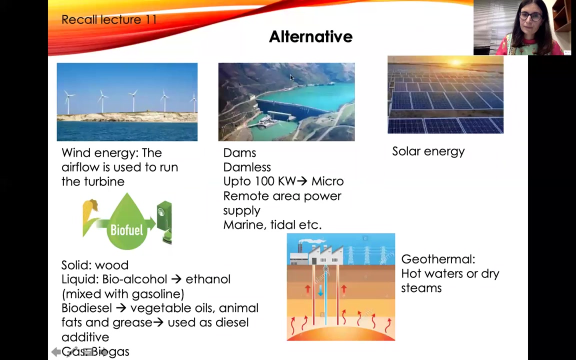 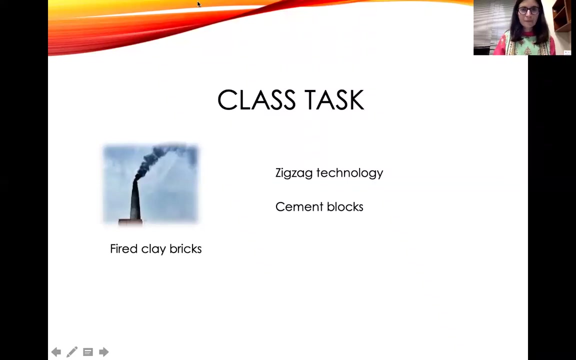 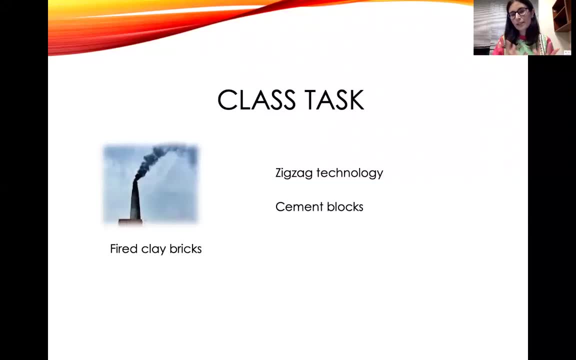 And yeah, so they're just placed straight in line. here You're allowing for it to zigzag, zigzag, zigzag and then finally go up. So, whatever heating process you're using, you're allowing it to be used and reused. 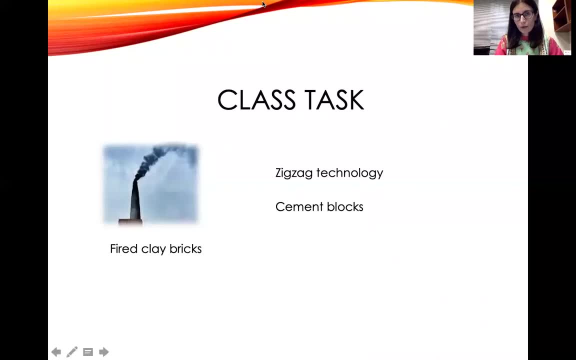 And then finally, it just emits out: Okay, The end of the pipe, Excellent, Right. So it took me a while to understand it, because I had to go and look at the design of a brick kiln and see what does it look from inside? 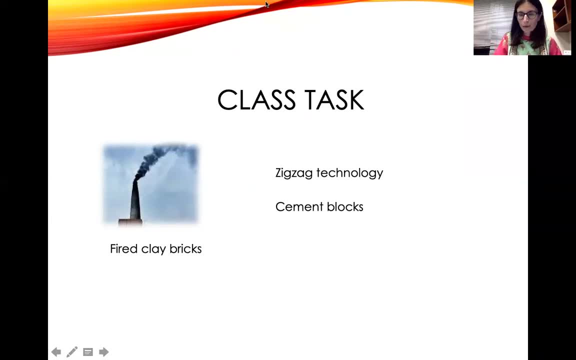 And then you know. then I was able to understand it, But you guys are clearly more intelligent. So if you get a chance to go to brick kiln again, I would definitely request you to just go in and see what's in there. 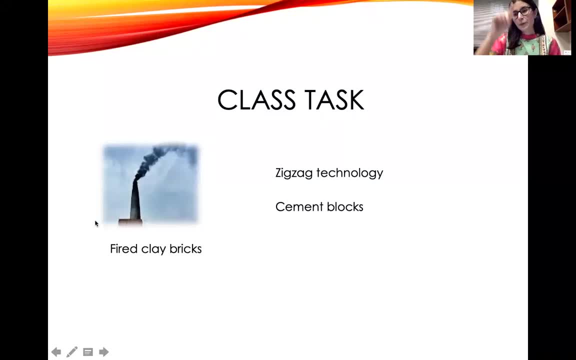 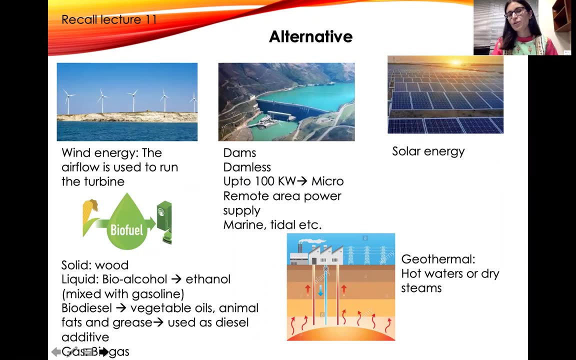 But yeah, so basically we're trying to cover All the sources of smoke that we mentioned in one of our initial presentations. Here, I think we should definitely mention what is the alternative to all the dirty fuels. We've already talked about them. 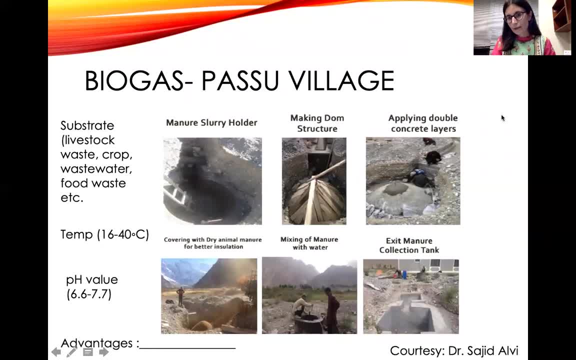 So I'll just highlight it. Someone has raised the hand. Aapka, is it you? Yes, I just wanted to add something. Go ahead From the economic point of view, like I wanted to talk about this exact technology that you know. it is said that the return on investment. 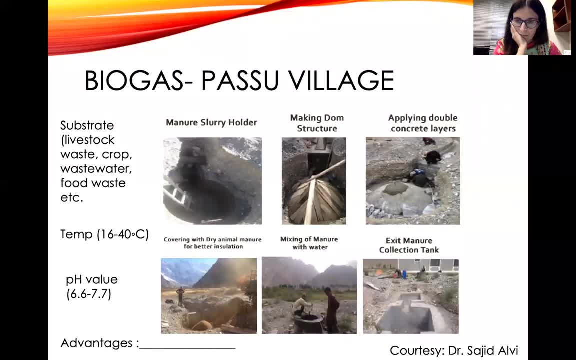 Yes, Yes, It is said, when using zigzag technology, it can be achieved within a very short period of time, And in Pakistan, because of small crisis and winters, especially like in Punjab. So the Punjab, what the Punjab government did, was that it used to just shut down the traditional brick kilns, which obviously resulted in millions of like a loss in millions of rupees. 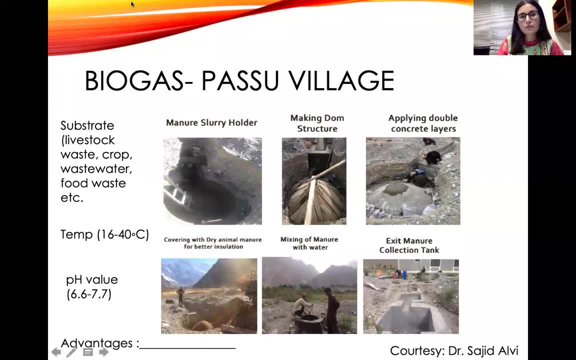 So with this particular technology, it is reported that the brick kilns are not as good as the traditional brick kilns. The brick kilns can actually run throughout the year as well, So you know it's economically very beneficial. Yes, absolutely. 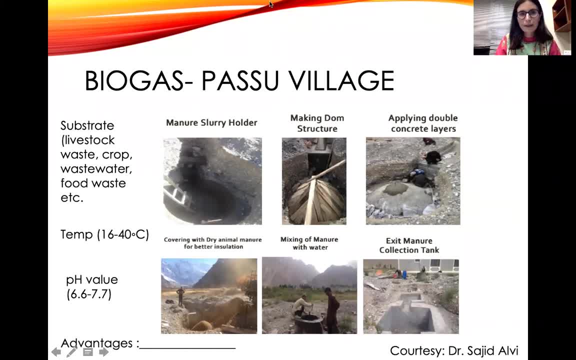 So thank you guys for going through the process and searching it and contributing to the class. Basically, we've also discussed something else, which is biogas, And biogas is a mixture of methane and carbon dioxide. We use it, but we can also kind of prepare it using oil. 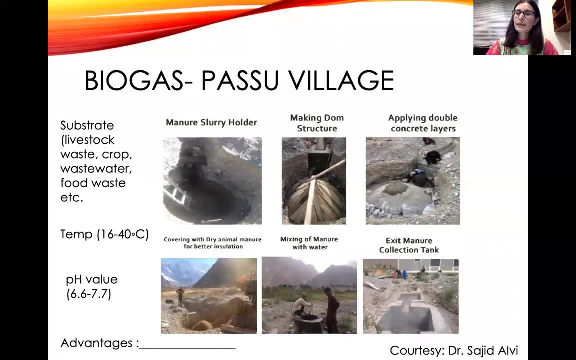 We can also use it in our waste food, And this particular case study I came across recently. it's also done by a student who is now a doctor in one of the villages in Hunza where he basically used that. Of course, you study the advanced designs in school. 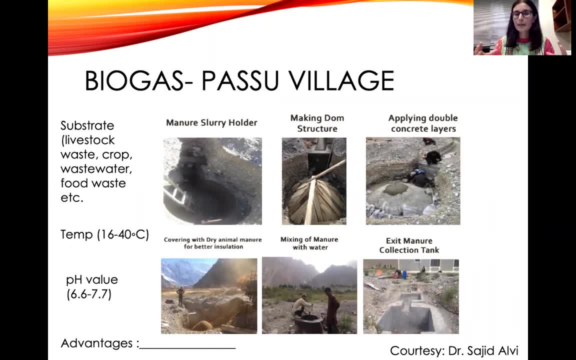 But when he went there he used all of those principles, built that setup allowed for the slurry to leave, created that dome shape allowed for a pipe to leave. And then you know he's written all of his optimized conditions. 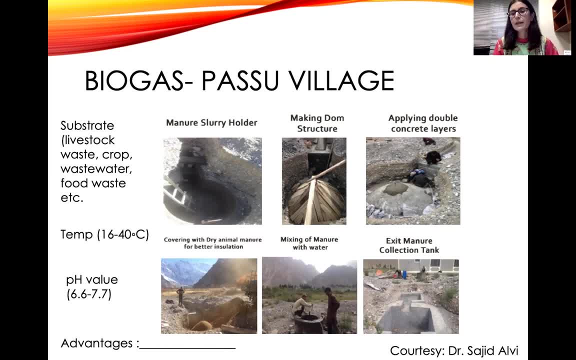 Like: what are the temperature requirements, What were the PhD requirements? And at the end of the day, he was not only able to get gas, but also the waste that came out was fertilizer, So biofertilizer for his crops. So yeah, I found it interesting. 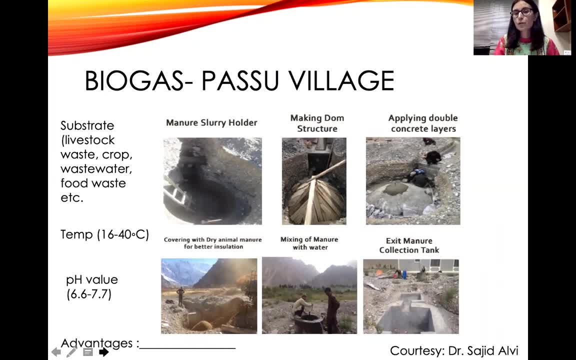 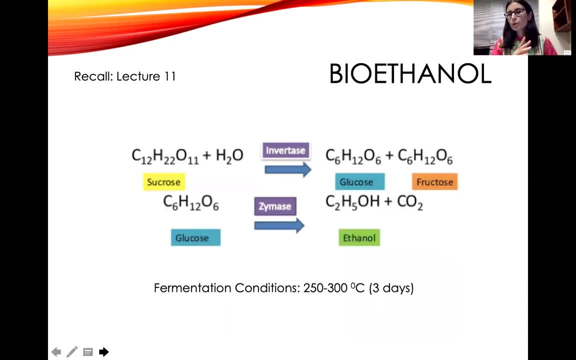 And then I thought I'll share it with you Again. we're talking about alternatives to fuel, And you know we've mentioned it, so I'll not discuss this in detail, And this is also recalling your lecture- It's 11, where we looked at bioethanol, which is another liquid fuel that can also be used as a cleaner fuel compared to fossil fuels. 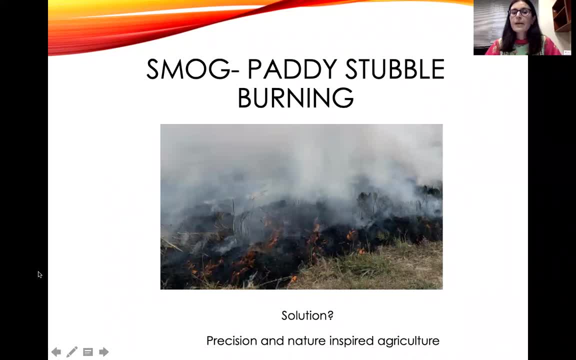 And lastly- I hope this is lastly- we also said that. you know, of course we said that some of it. we say that comes transboundary, which is why I want to just discuss how the weather patterns would change the flow of particulate matter. 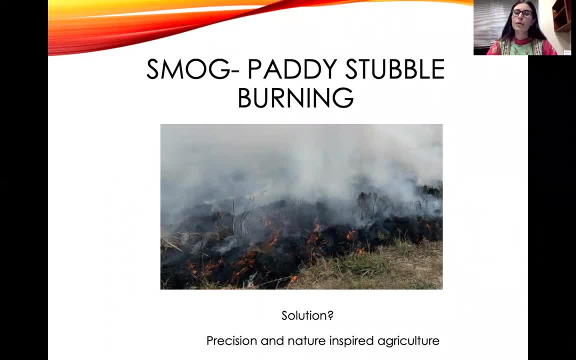 But I'll leave that for today's class. We are burning the paddy fields. What is the solution? And you've all discussed it and I've kind of given you a hint as well. Can anyone raise their hand and tell me how would you reduce the waste, not just smog, but also all other particles that are coming out of agriculture? 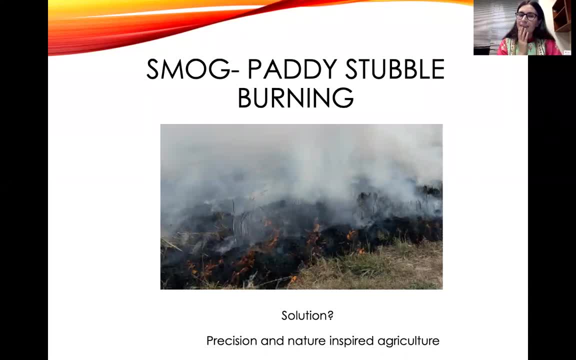 Anyone remembers. So basically you harvest the rice And then whatever remains because it's hard to take out, they just burn it and then kind of make it, make that a part of the soil again, and generally it is found to be useful for the soil. at least some farmers find it useful for the soil and it reduces work load for them. 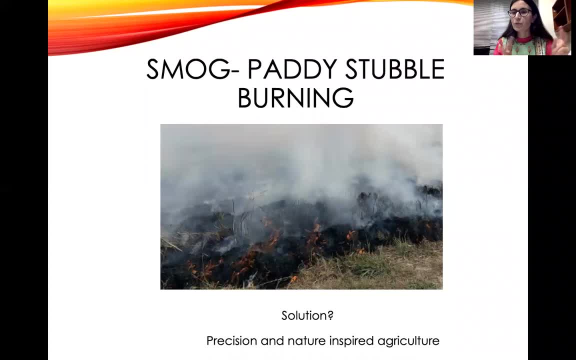 But this has been. this has been mentioned as one of the biggest sources of smog in Delhi and Lahore, and this, this area as well. So who knows what the solution is, And we've discussed it in four lectures, in different lectures. 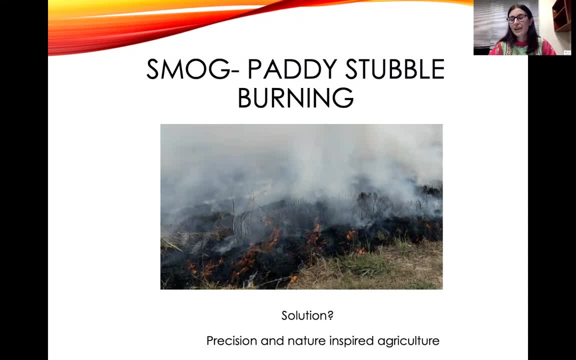 So who knows what the solution is, And we've discussed it in four lectures, in different lectures, All different ways. Rafee, did you raise your hand, Or was that? Yes, go ahead. Oh, I raise my hand. 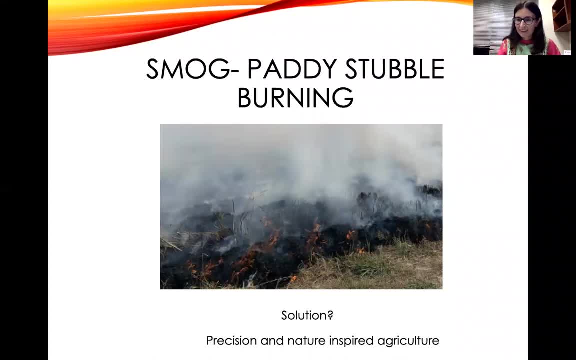 Nadia mentioned mulch and I was about to say, and also that you know, when you ask that, are you asking, how are you asking about transboundary pollution? No, I'm just asking. Let's say there's a rice, So there's something that we've talked about a lot. 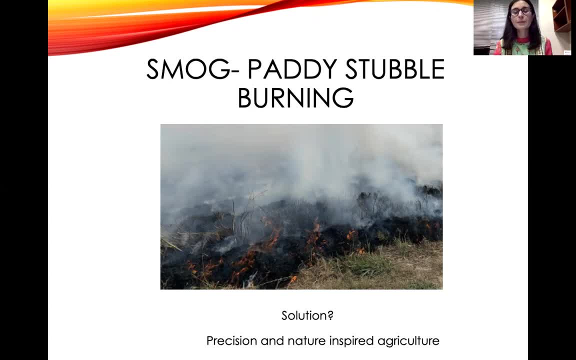 farmer also said so. mulchings covering the soil, yes, but this soil has remains of a product in the soil, and now they want their soil to be suitable for agriculture again. um, there is something that we discussed in the agriculture that i don't know why i'm forcing you guys to remember it. 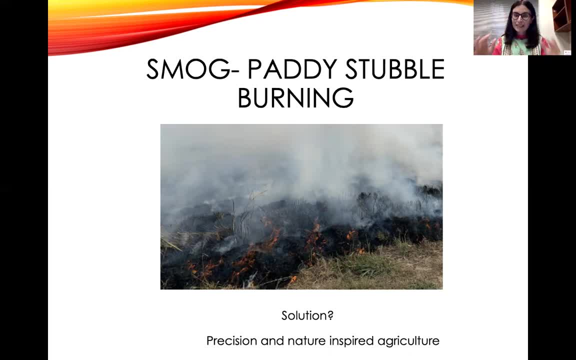 do you? okay, you don't have to remember it. so, basically, when we said that the sustainable or nature-inspired agriculture aims towards no-till technology or zero till, and that we are not, which means that we're not using a tractor or something else to kind of 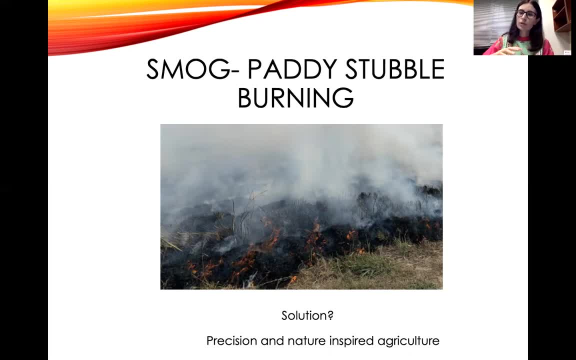 uproot the soil and uproot the plants, or topple the soil and uproot the plants. we're basically just allowing for the. you know, whatever we're using, we're only using it to put our paddies, or fresher paddies, or seed in it, and we don't take the older crops out. 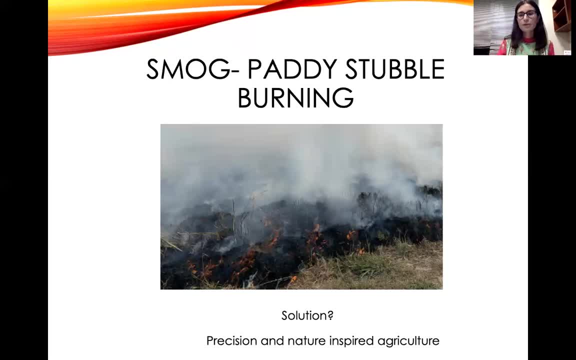 and then they just decay naturally and become a part of the soil, so you don't have to burn it, which means that what you've studied in agriculture also has a role in air pollution, and i just wanted you to make that connection here and um, and yeah, i mean you can, you can look. 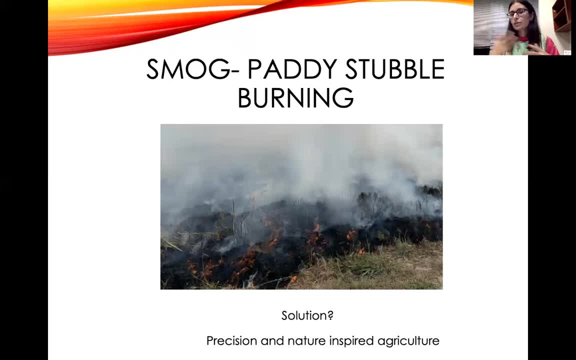 at it at various ways: composting, yes, using fertilizers on source, yes, but like in. in terms of agriculture, i think it's zero till or not, which was a part of, you know, the sustainable agriculture, and now it's growing. so we, we said it already started in the 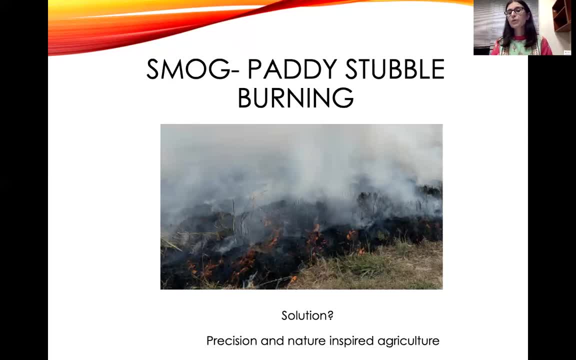 90s and 70s. the only thing that's shifted is now you're using tractors that are only putting the seeds in without disturbing the overall soil, because they are carbon dioxide sinks as well, and when you try and irrigate it, when you disturb the soil, all of the carbon dioxide 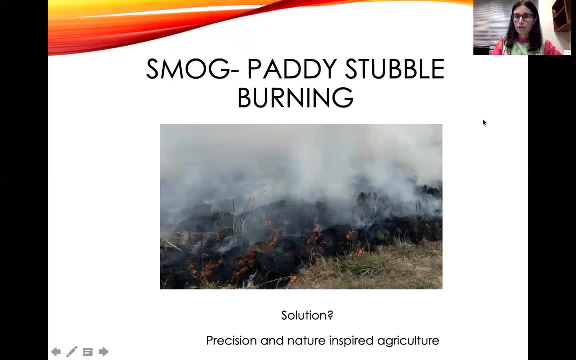 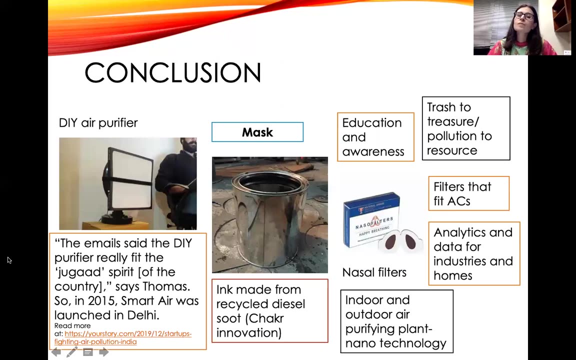 is released back into the atmosphere. nadia has a question. what a point uh, ma'am, uh, there's a previous uh talk uh from, uh, from uh the group. you said that people should not take out the residual of the previous uh crops. but, ma'am, there must have been some advantages. 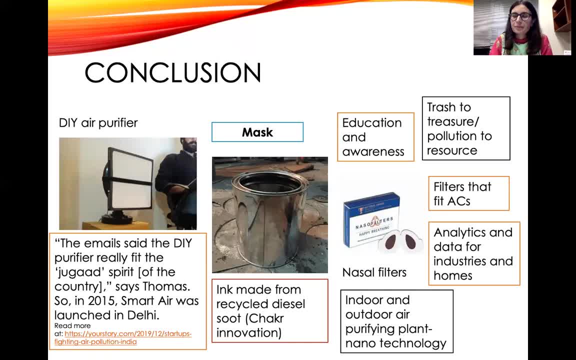 of taking the residual of that plants right, otherwise why would they take on such a hard working task in order to- i mean, for their cultivation or agriculture? yeah, so basically, it's convenience, nadia, and it's factory. you know what i was saying? it's monoculture, and if you want the machines to do that for you, you just disturb the. 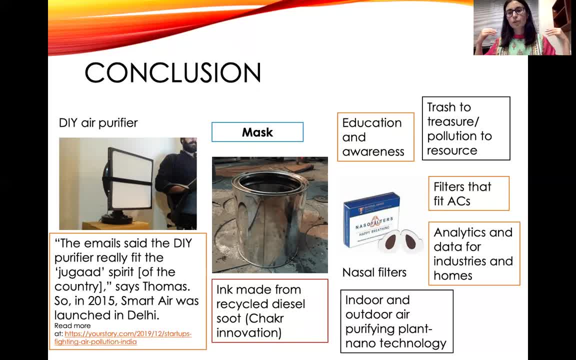 soil, use the same kind of equipment, use the same kind of seeds and then irrigate or practice agriculture or a longer space of time. but if you're more considerate of the environment and, like I said, when you disturb the soil, the soil quality decreases, because we said that the top thin layer has all the 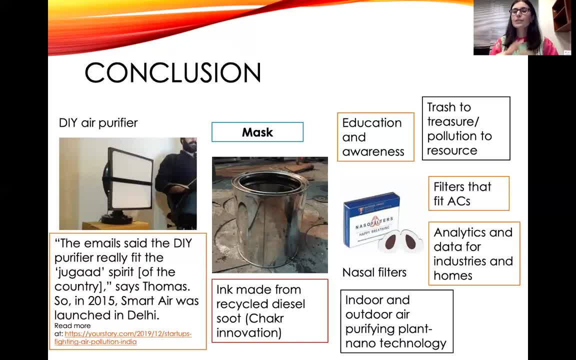 beneficial microorganisms and the beneficial nutrients. and you know, most of the compost lies there, lies there as well, or most of the peat lies there. so if you disturb it you're kind of also disturbing the life that's inside it. but apart from that, the carbon sink that is created, the carbon that was stored in, 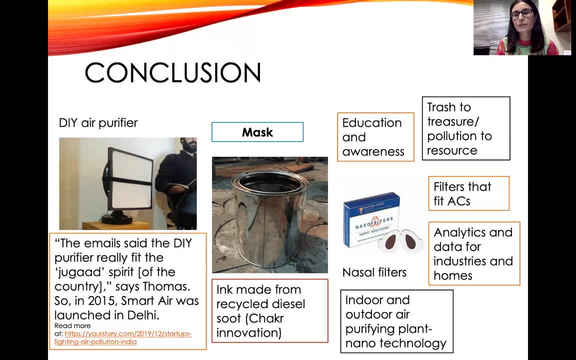 the soil oxidizes and it is released back into the atmosphere and and so it is multiple disadvantages. what we looked at with the farmer, with nature inspired agriculture, was the fact that we don't need to do this. we all we need is for the soil to just go in and you know, and be able to grow the rest of it can. 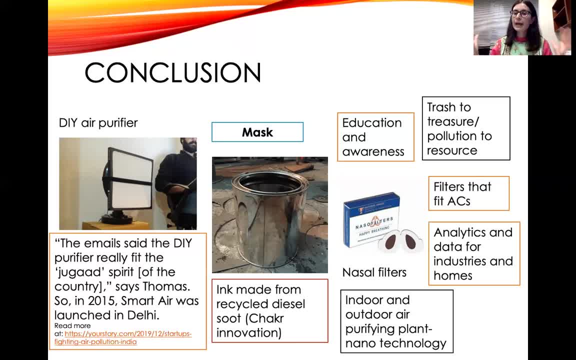 naturally decay and become a part of the soil and can also act as a not only best reducer but also a cover for the soil. and on top of that, the roots, when they go into the soil, can be, you know, can penetrate and provide extra space for life and oxygen and nutrient or water absorption into the soil. now the 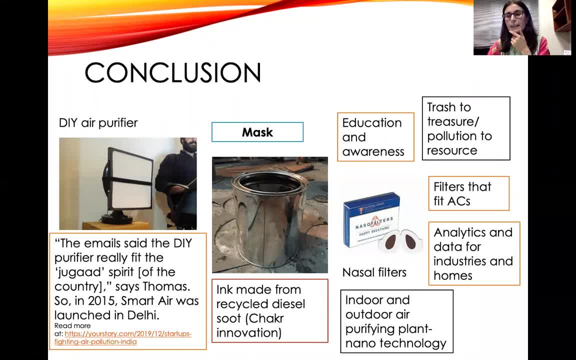 problem with soil- rice paddies. soil has also beenстрated. sorry- is that they are hard to take out and that's why they burn it. if they were easy to take out, they wouldn't. they would probably just take it out. but it's hard to take it out and that's why. 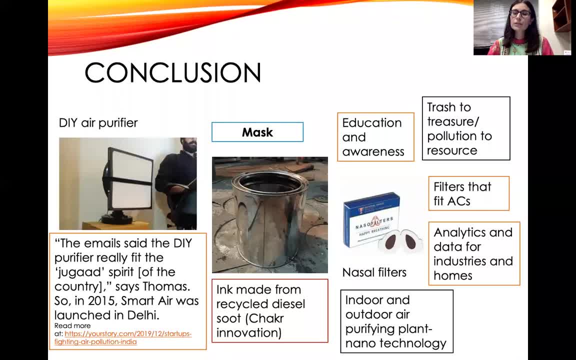 they burn it because it's easy, but we know that burning has consequences. i think we need to change the practice, and the practice part is what we had discussed in the agriculture- that whatever we are talking about, it wasn't just limited to agriculture and biota and natural environment. 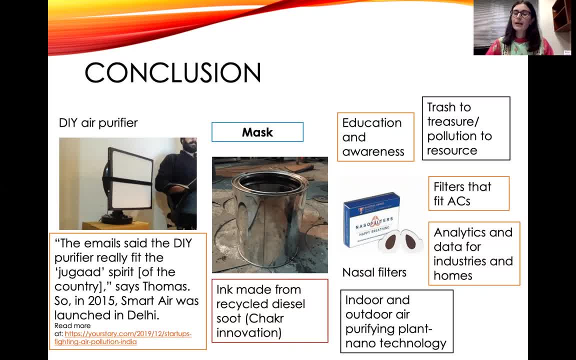 but also the fact that these practices could then keep our air clean too. so again, those multiple actions with with nature inspired practices. how much time do i have? one minute to conclude the lecture? uh, if you bear with me for another minute. so basically i was just looking at quick startups. 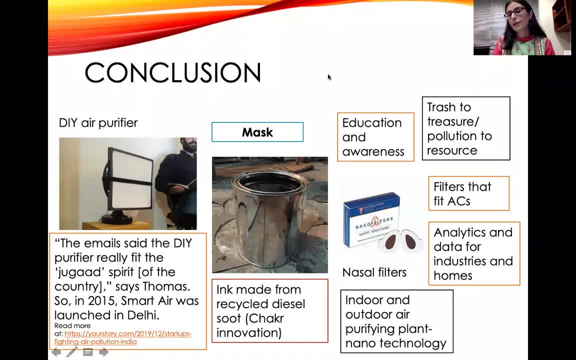 and i found a lot of stuff, startups from india, and that's maybe because they also have a lot of smoke, uh. but basically, uh, there are these. this one i really liked, because they also call it the jugard purifier, because the guy who developed it was, of course, a foreigner studying in china. 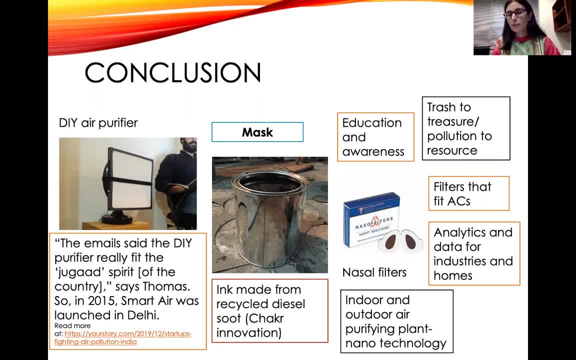 and when he found out that the purifiers are the air profiles are really expensive, he found out what's in it. it was a hepa filter, which is high efficiency particulate air filter, a finer filter. he just put it with his normal fan and that basically acted as a 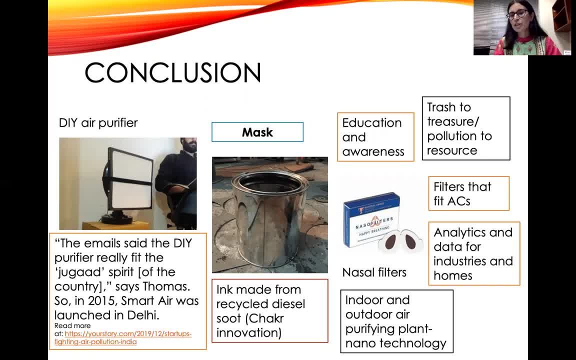 purifier for him and he then is. now he commercialized it and he's selling it. and, similarly, there are many, many startups that are using the suit or that, that carbon that's coming out from diesel, from other practices, to make high quality ink, high quality paint, etc. so, basically, 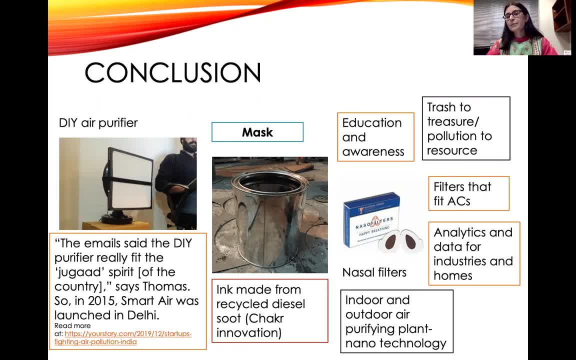 reusing the source. there are a lot of other startups that are creating education and awareness, startups that are giving the industries the data and analytics of the air quality, like you know, big companies like microsoft, ymca- all of these are well known and they have the opportunity to make their own products, but they have a lot of work in the industry. 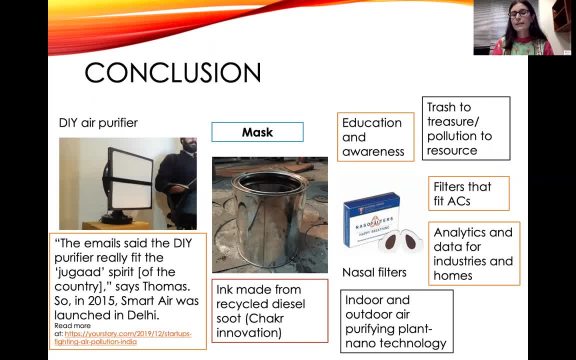 so many startups are using the same technologies in their brand. you will see in the in the first part of the video i'm going to show you some of the other programs that, uh, they have, but both of them have a lot of contributions to their business and also they're using very 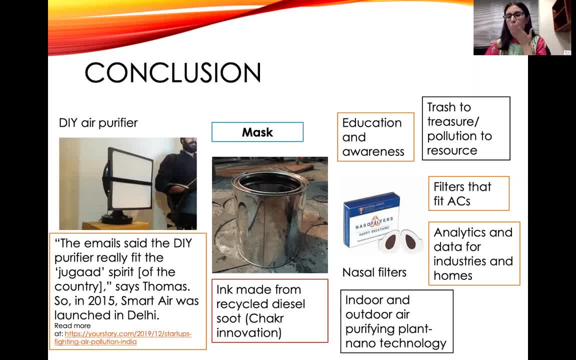 much their creative work and they're creating their own tool sets, um. so the first one is the um, um, these small interventions which, of course, must have taken for them a lot of time to develop these basic prototypes. but i just also wanted to think outside of industries and vehicles, and 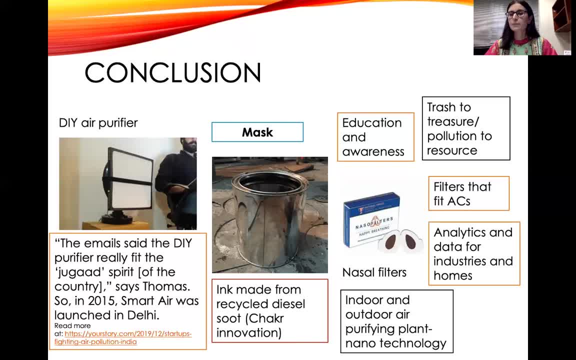 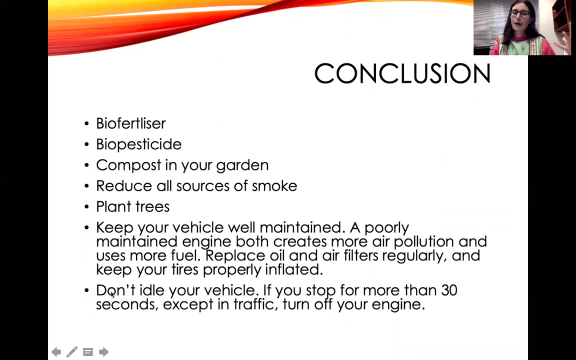 agriculture and all the normal things that we've generally discussed in the class, but also think about others. and, of course, uh, plant um as, as eminent said, life. so uh, pure air purifying plants, inside the house or outside the house, across the roads, whatever. they will also improve the environment. and bio-based things: biofertilizers, biopesticides. 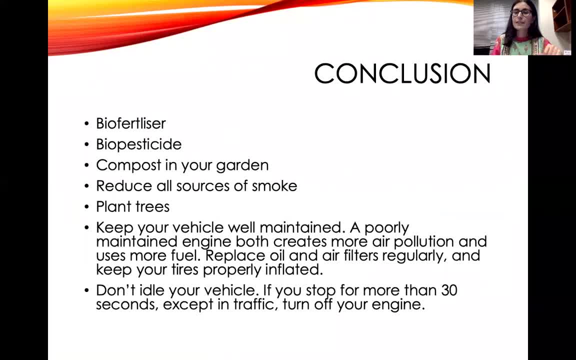 composting in your house, keeping your vehicle regulated, changing the oil, cleaning the filter- but changing the filter as well- and then making sure that your vehicle isn't sitting idle, because it's said that a lot of the emissions actually come from the traffic light time, so that time where they're waiting rather than the time where they actually 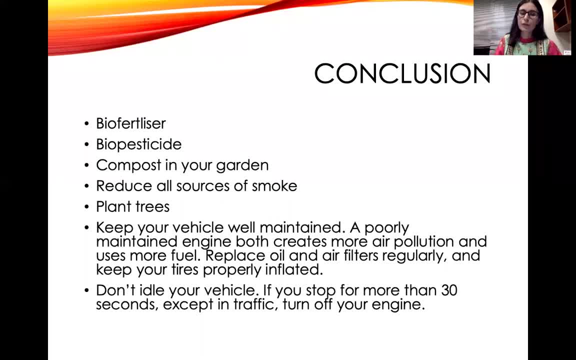 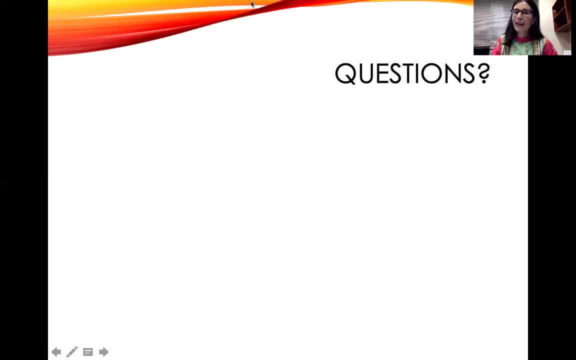 travel, so there's a lot of stand-up time. that costs us a lot of pollution as well. so just some of the things that i wanted to highlight. i think that's it from me. if you have any questions, you're more than, or comments, you're more than welcome to make it now, and meanwhile i read comments, hassan. 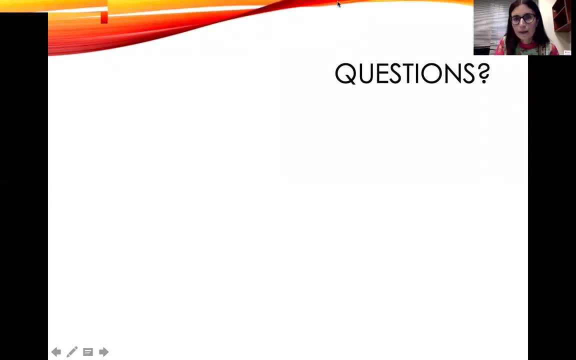 i just wanted to make a comment. where we previously talked about electric cars and how, in the long run, they would reduce emissions, but the fact that you just talked about signals and how the waiting time takes a very long, you know, a very long time. tesla currently is trying to. 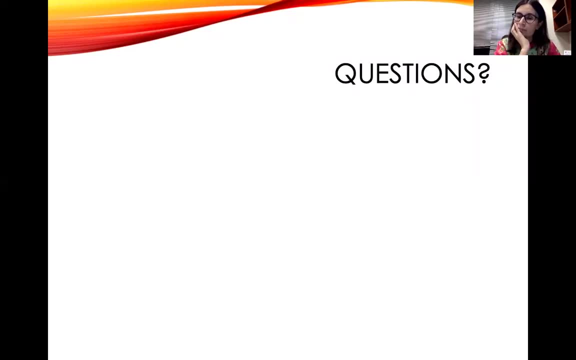 implement something where there's basically a mesh of cars and each, every car is connected in the network. so, uh, before even reaching a junction, the cars know, uh, which other car is approaching, so they adjust their speed in such a way that it minimizes the waiting time. so they 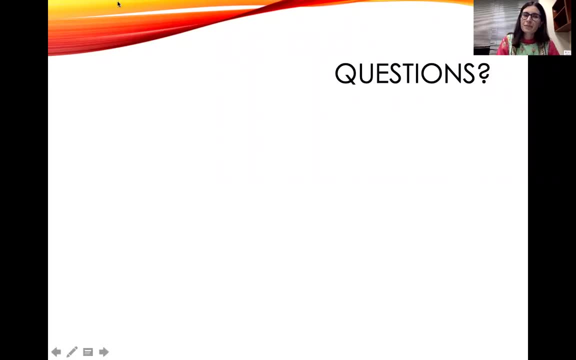 can just pass by each other without ever colliding and they don't need any waiting time at all for signals. yeah, yeah, yeah, i mean, of course there are a lot of narratives, but i think, yeah, i mean it's interesting that you guys think, think about those things as well and those interventions as 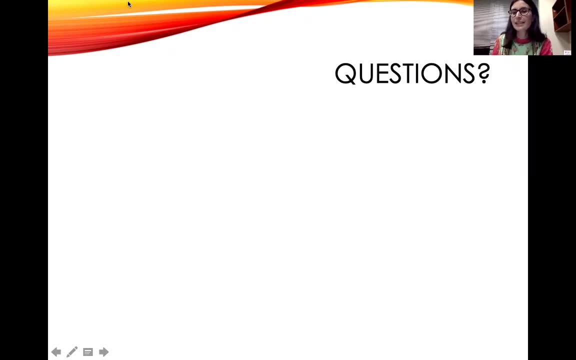 well about how these cars can also be designed smartly to operate. in any case, the car is not going to pollute. you know it doesn't have end of the pipe. so remember, we talked about end of the pipe for factories and brick kilns. an electric car doesn't have a pipe, it just has a battery. 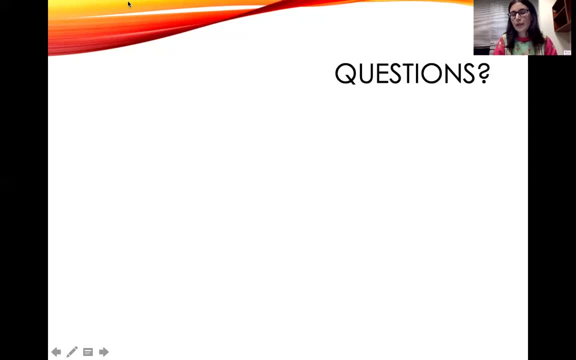 you know it's, it's like your mobile phone it does. it's not going to have a an emission source, but it might have indirect emission sources based on where the electricity is coming from and, of course, that's the biggest question. so, but a lot of people still say that even after that, because the the 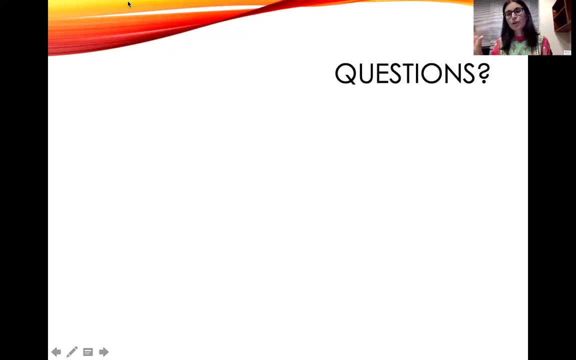 fossil fuel run cars are less efficient and the electric cars are not, um they they might still benefit the environment more and of course, because i i want cleaner technology to come in. so i'm a pro ev. but you know there are all kinds of narratives and and some that makes sense. so depends depending on which country you're in. 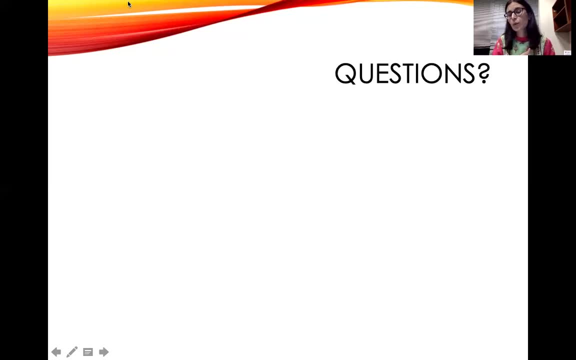 so, for example for pakistan, we might be using the dirtiest coal for for developing electricity. and if that electricity is going in into the electric vehicle, if that electric vehicle is going in to a fossil fuel run car, i would still believe that because that fossil fuel car has end of the. 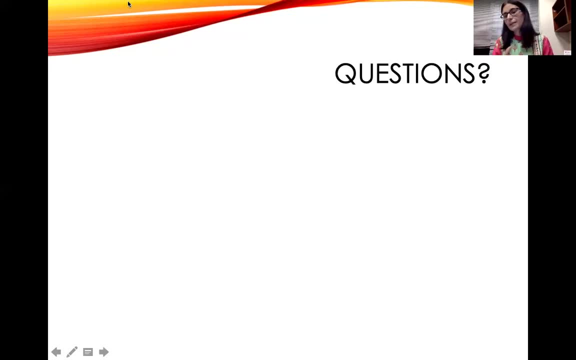 pipe. it would probably be better than that. and and of course, there are scientific like this in researchers and numbers and and data analysis that shows that and i want to believe it. so i do believe it. but yeah, did i actually i? i understood your point right. did i mess that up? 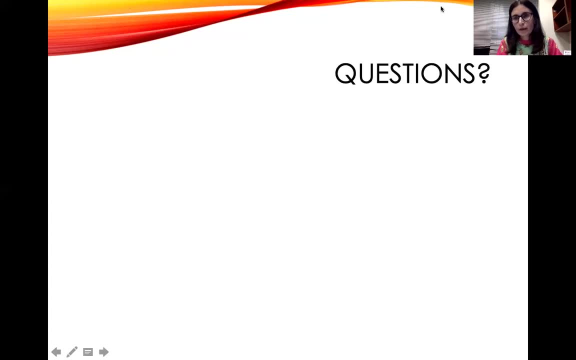 did i mess up what you wanted to say? yeah, that's right. okay, it okay. thanks, husband. anybody else? i just need to send a private message to some people. i want to stay back. any other comments, guys, before we leave? no, okay, nadia, do you have a question?